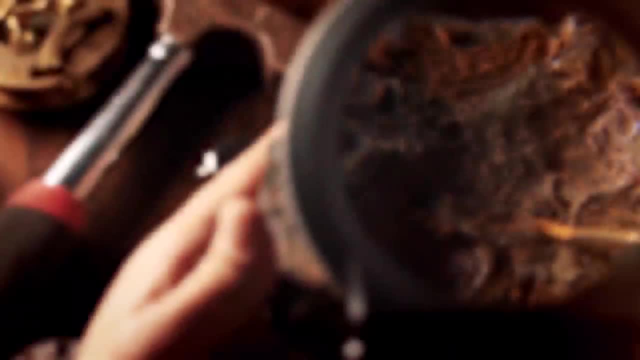 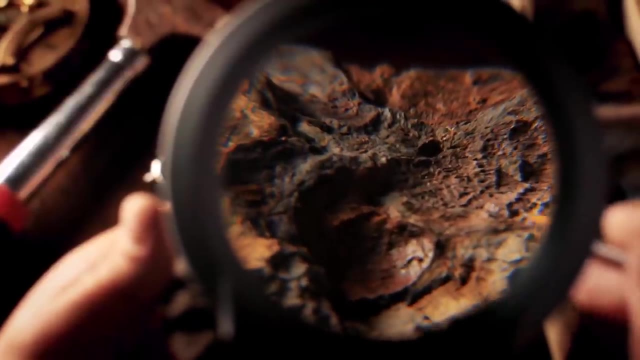 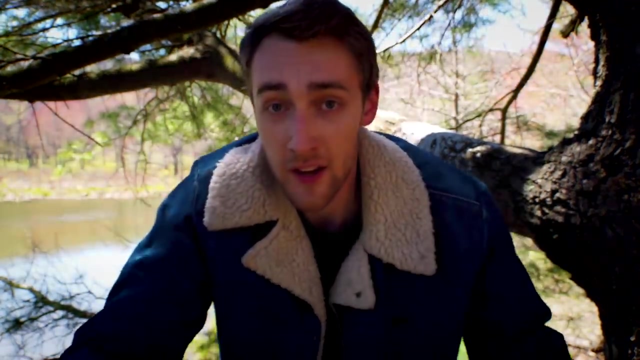 are still piecing together to this day. Because of this, our knowledge of dinosaurs can never truly be considered complete, But we can definitely use the picture that's emerging to better understand how life on Earth has progressed to get where it is now. But here's the problem: I don't actually know that much about dinosaurs, I mean. 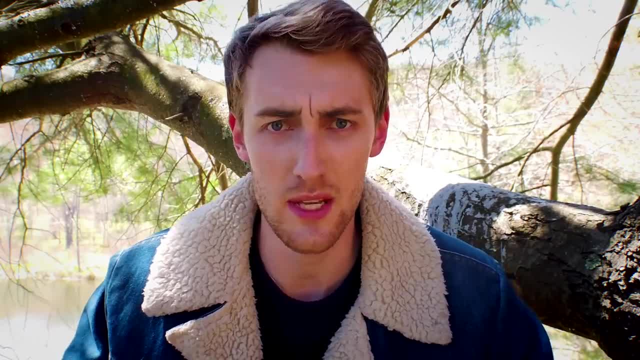 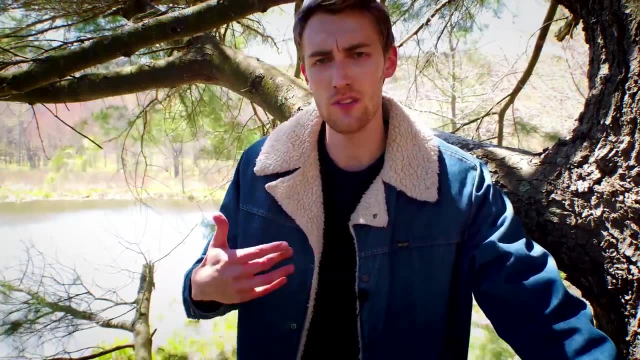 even as a kid, I was never really interested in them, As it always just seemed like memorizing a bunch of different animals without any sense of why it mattered or how it even related to today. When I got to college, I was taught to think in terms of systems like Earth systems, ecosystems, climate systems, 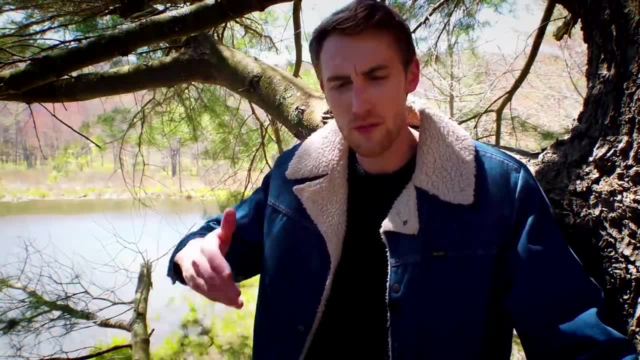 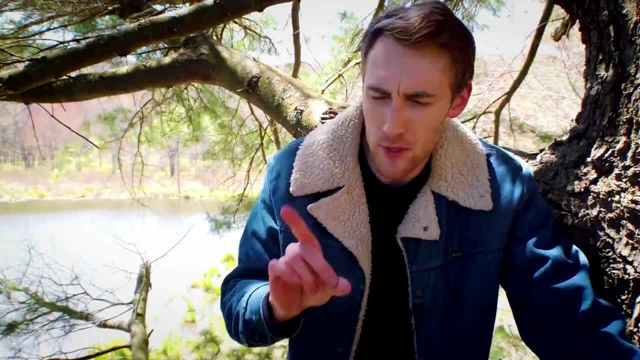 planetary systems, whatever, And so learning something without any sort of framework, like learning all the different sorts of dinosaurs, always felt less like knowledge and more like information, if that makes sense. But you know what, Now that I've been through college, maybe it's time that I look for the underlying structures of dinosaurs myself. 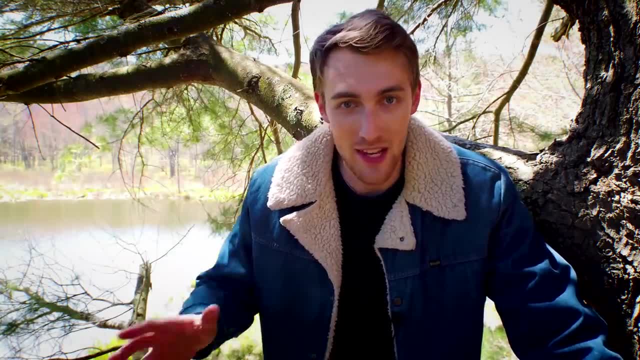 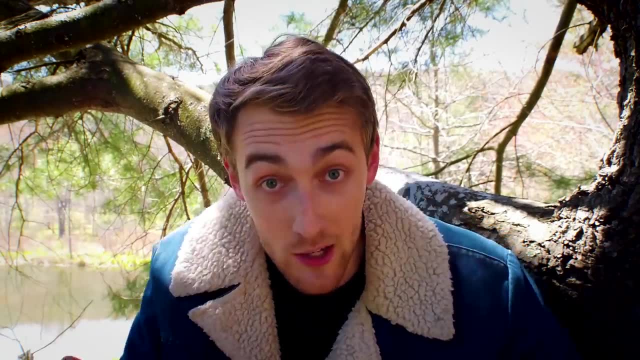 After all, dinosaurs are some of the most utterly amazing animals that have ever walked this Earth, And so I'm sure if I just understood them better, preferably through something visual like geography or, even better, biogeography, then I could really learn to appreciate them. 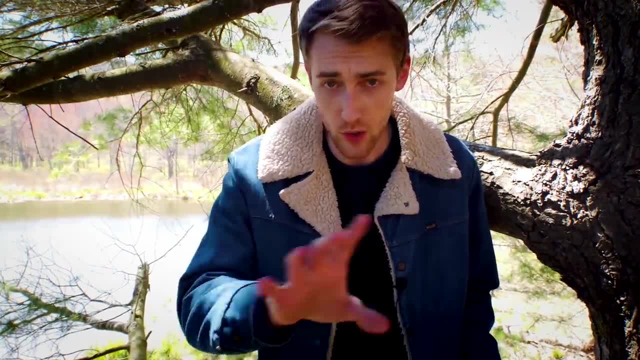 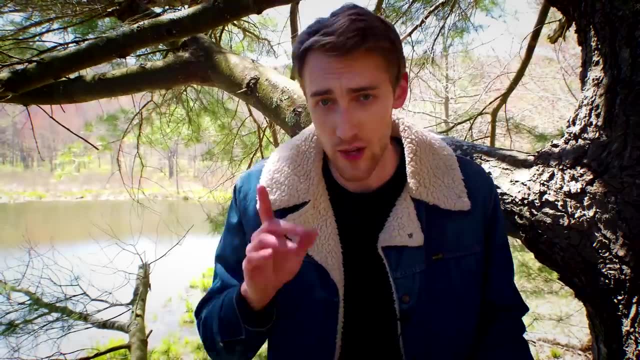 So that's my goal for this video: to build, for myself and for all of you, the basic framework to understand these creatures and their evolutions, both over time and across continents, So that, going forward, I have the knowledge to make more videos on these wondrous creatures that were the 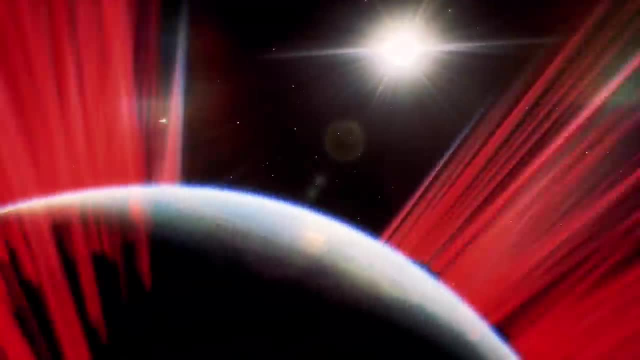 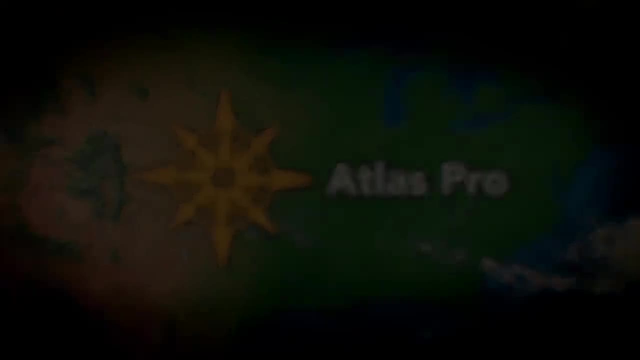 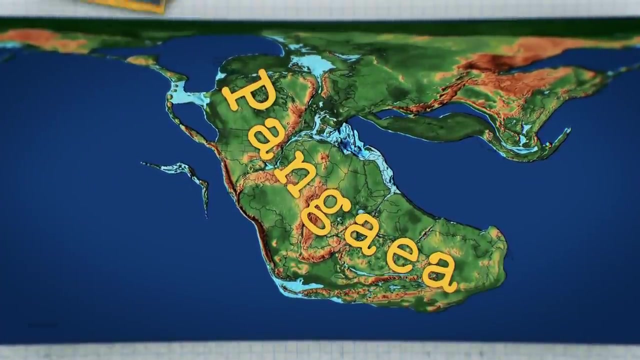 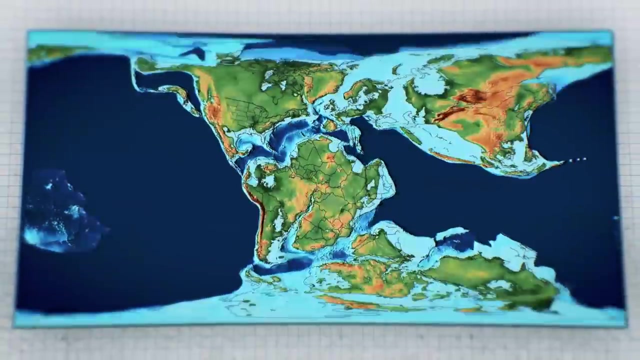 dinosaurs- INTRO. The story of the dinosaurs starts over 200 million years ago on the supercontinent Pangea, As I explained in my 7 Realms of Biogeography video. it would be from this landmass that the continents of today, and, by extension, their distinct flora and fauna, would later all. 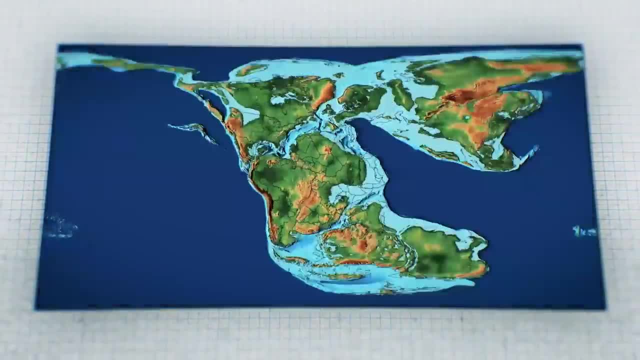 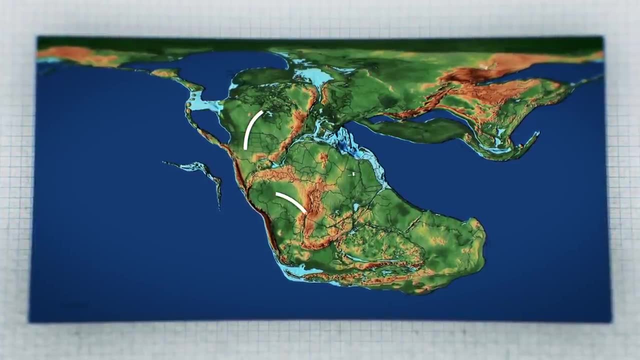 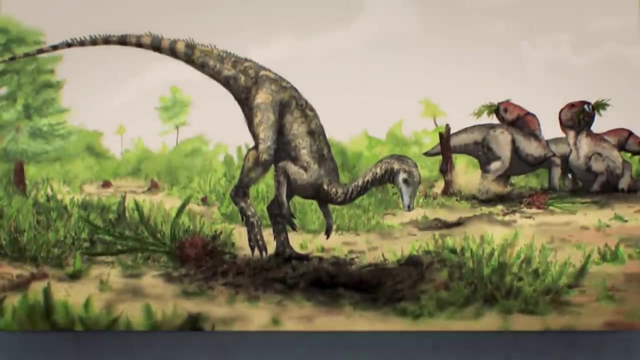 delineate from. At the time, however, Pangea's connectedness allowed for a more even distribution of species across the planet, resulting in one unified global plant and animal community, or in other words, just a single biogeographic realm. While the earliest dinosaurs may have emerged as early as 240 million years, 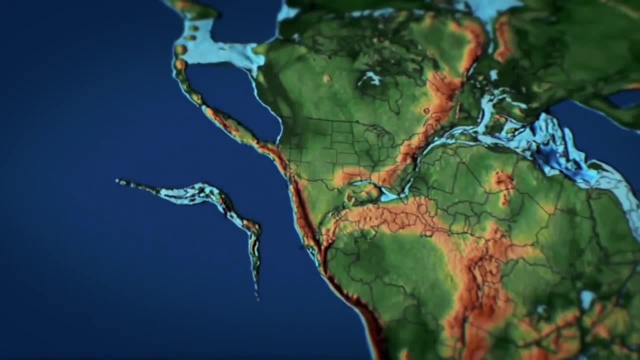 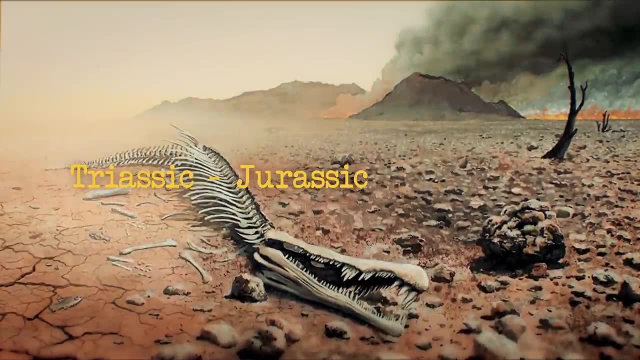 ago. at the time, the dominant creatures of the Earth were massive amphibians like Temnospondyli and large reptiles like Phytosaurs, And it wouldn't be until the Triassic-Jurassic extinction event, around 200 million years ago, that the dinosaurs would be able to make their way across the planet. 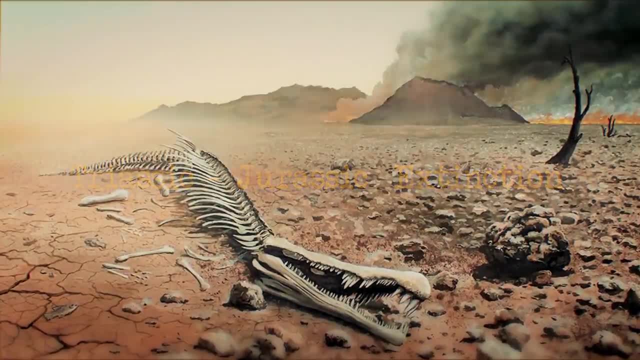 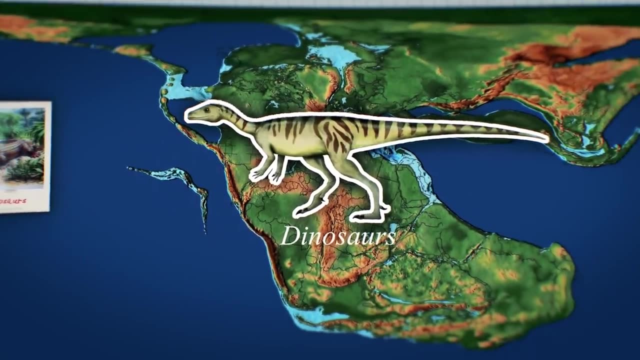 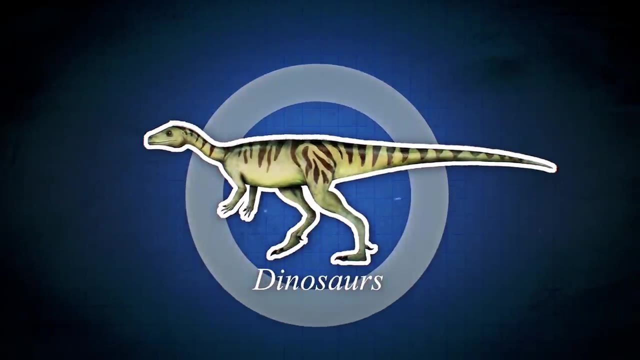 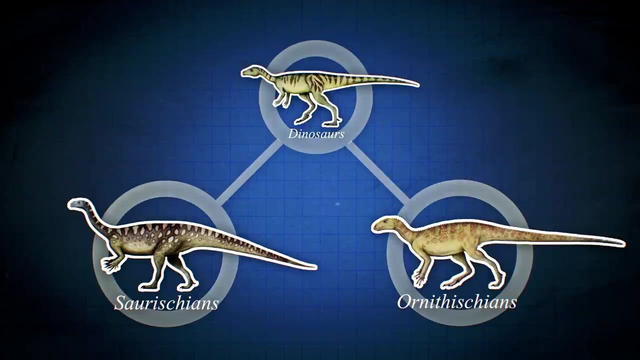 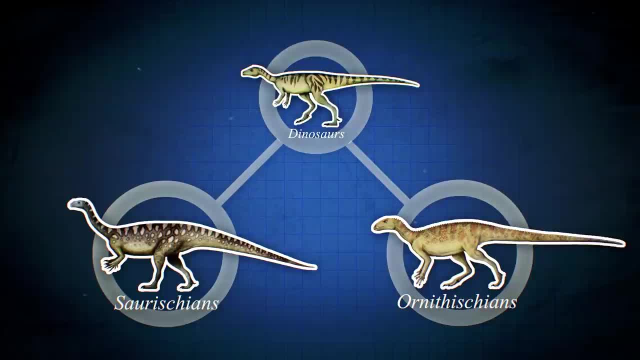 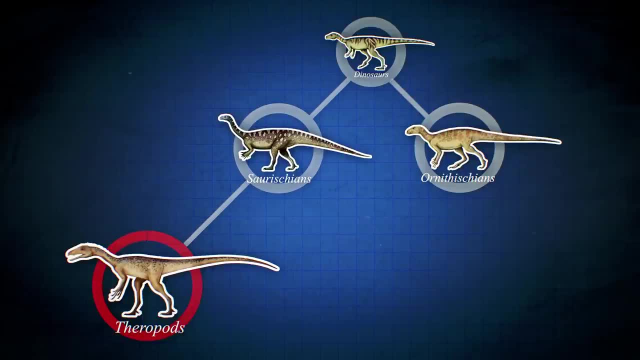 matter of time before a dinosaur came in to fill the void From the saurischians. a group known as theropods quickly diversified into a mainly carnivorous role, while what was left of the saurischians became the herbivorous sauropods, establishing. 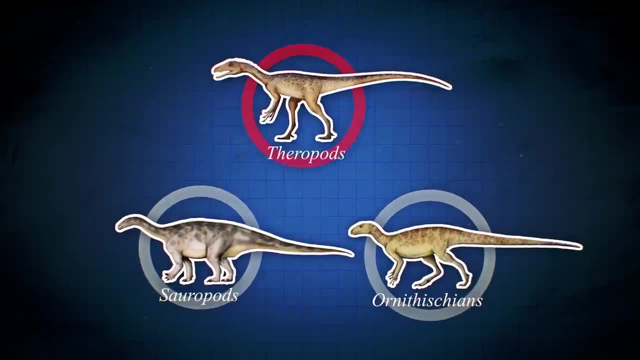 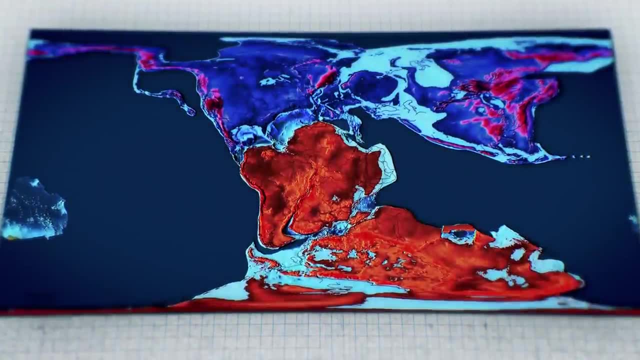 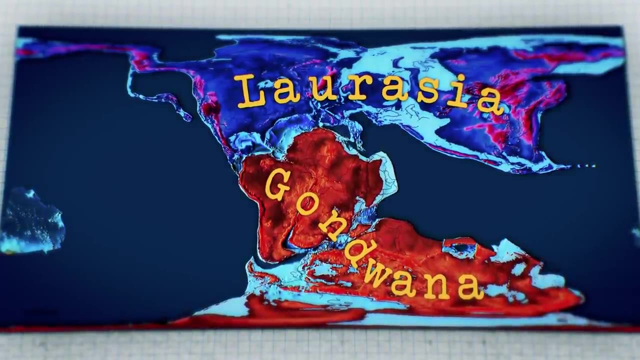 a single prevailing food chain across the whole pangeic realm. But, as we all know, pangea would eventually start to crack, with the first break coming in the division of north and south Laurasia and Gondwana. And as the divide between these two continents widened, so too did their animal communities. 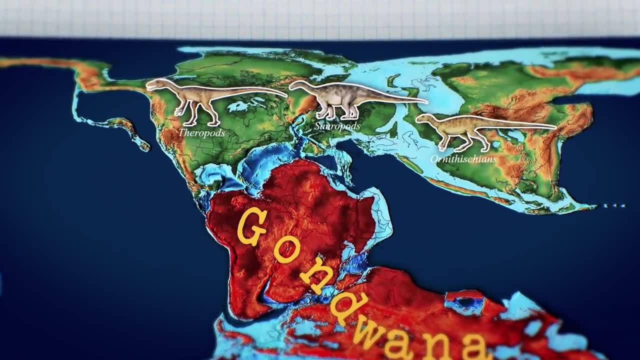 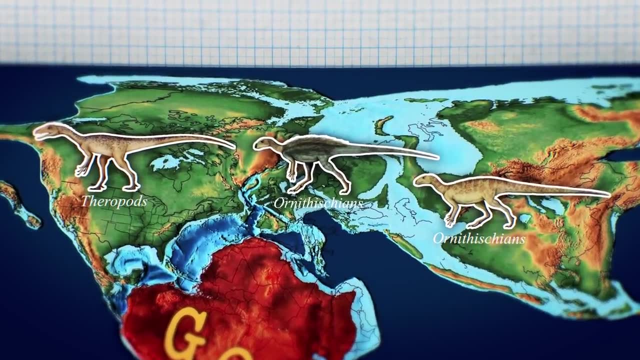 Across what's now North America, Europe and Asia. sauropods were mostly out-competed by the ornithischians, which gave them the space to diversify into a variety of forms. While I definitely can't mention them all, some of the most common, both in the fossil 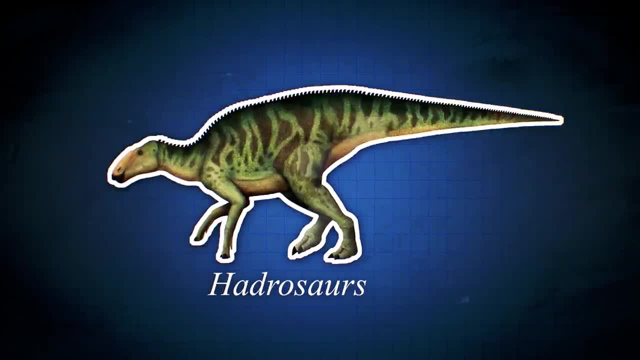 record and in media would be hadrosaurs, or the duck-billed dinosaurs which I've heard described as the cows of the cretaceous Iguanodons, which, to be honest, I don't even know what they are. 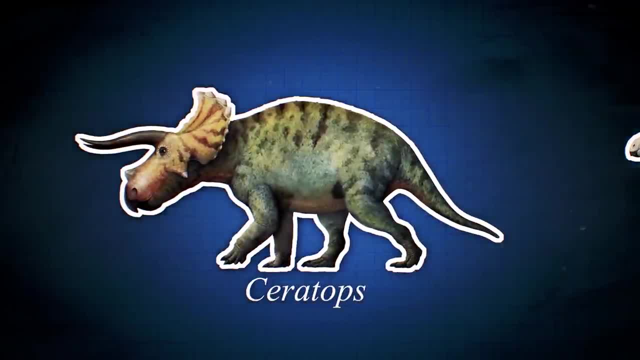 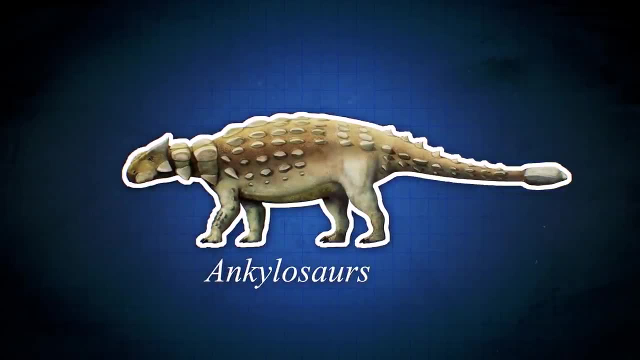 They're more of the basic dinosaurs: ceratopses or the horn-faced dinosaurs, I guess, making them the rhinos of their time. ankylosaurs, the absolute units of the dinosaur world which grew hard plates of armor on their exteriors, and pachycephalosaurs, or the dome-headed. 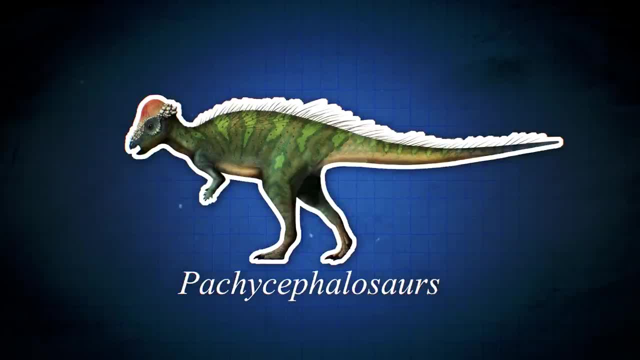 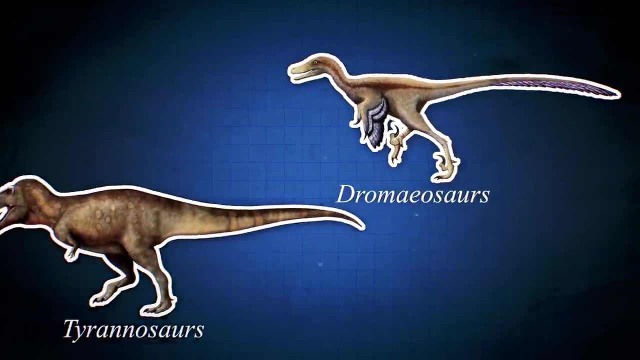 dinos, using their thick skulls, presumably to battle one another like mountain goats of today. Laurasian theropods, on the other hand, branched off into dromaeosaurs and tyrannosaurs. Contrarily on Gondwana, it's the same thing. 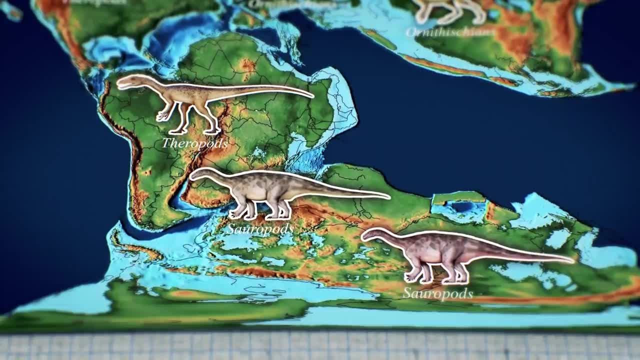 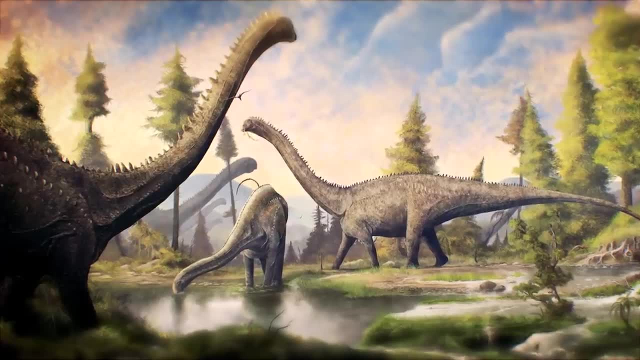 On Gondwana, it was the sauropods that came to dominate within the herbivorous arena. However, unlike the ornithischians, which developed into a wide range of body shapes, sauropods took the more if-it-ain't-broke-don't-fix-it approach and mostly maintained the same basic. 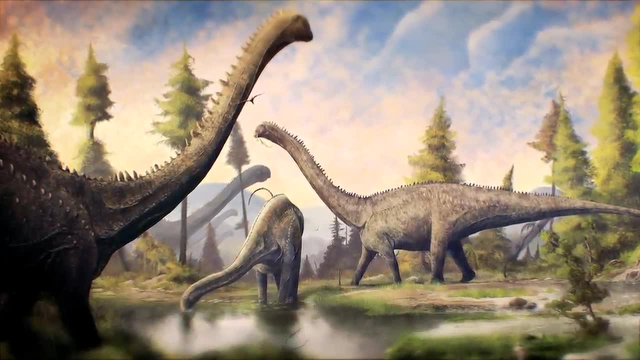 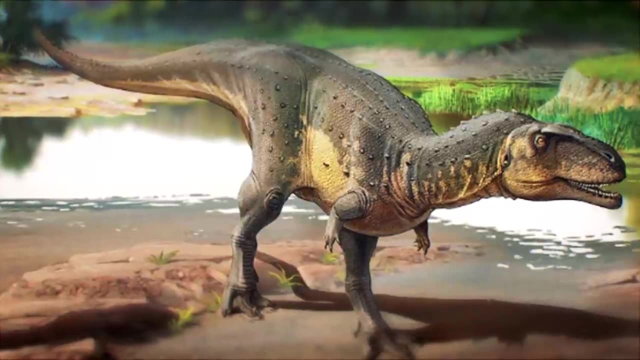 structure across all the different species that arose from this group, no matter how diverse they became. The same can be said about the theropods, which, despite branching into abelosaurs instead of tyrannosaurs in Gondwana, appeared virtually identical to each other. 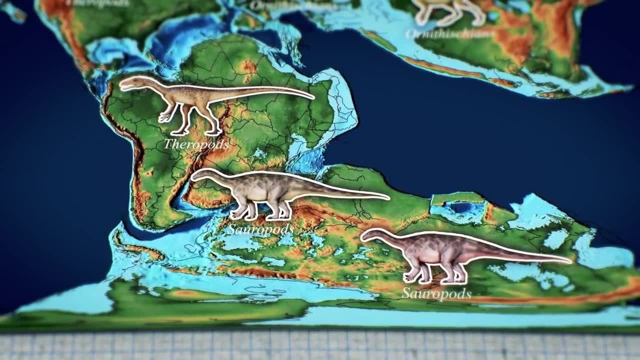 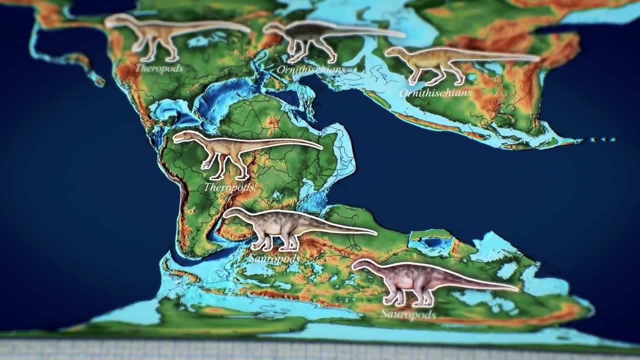 They were the same species but with a different structure. Overall, this left Laurasia with an apparently diverse array of ornithischian herbivores and Gondwana with a seemingly less diverse herbivore communities of primarily sauropods, both still 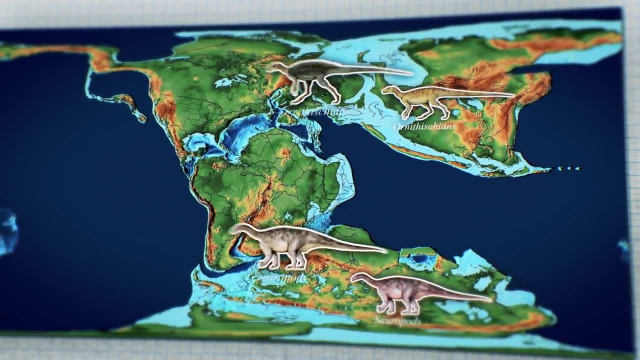 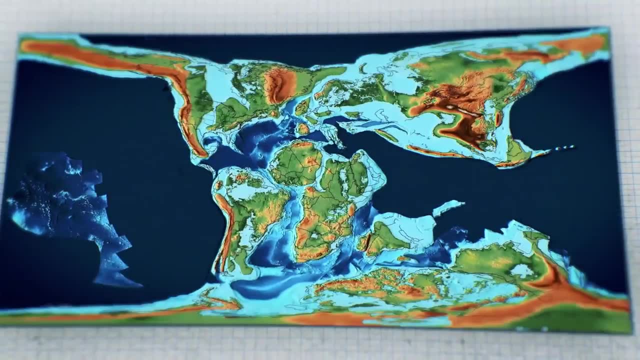 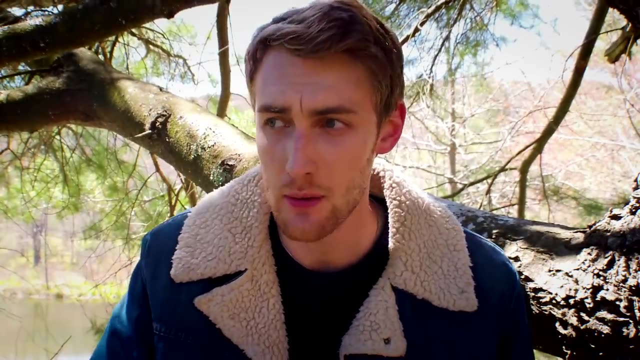 being preyed upon by theropods. These differences were only exacerbated by the continued fracturing of the lands at the dawn of the Cretaceous period, allowing the individual continents to begin developing their own unique dinosaur faunas. With dinosaur populations becoming more and more isolated, they needed to continuously. evolve in order to maintain their dominant status, causing their diversity to peak somewhere between 80 to 66 million years ago, during the late Cretaceous. Not coincidentally, this is the time period when most of the dinosaurs you and I are familiar. 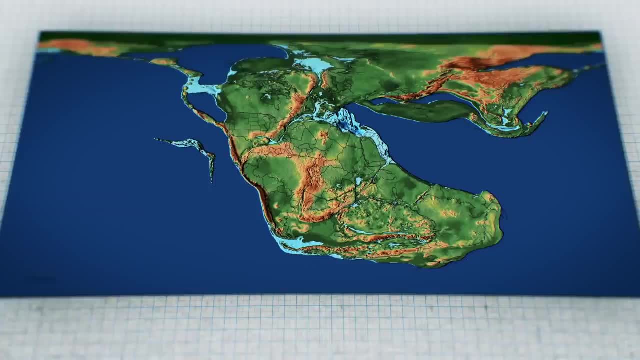 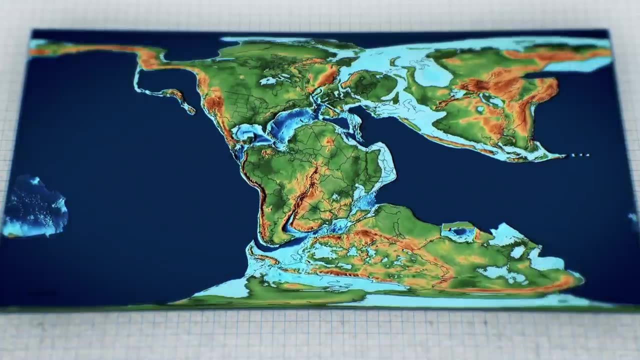 with roamed the earth, so that's when we're going to be focusing on. Although no single map can represent the earth over a span of twenty million years, to make things simple, we're going to pick just a single frame from this animation to represent: 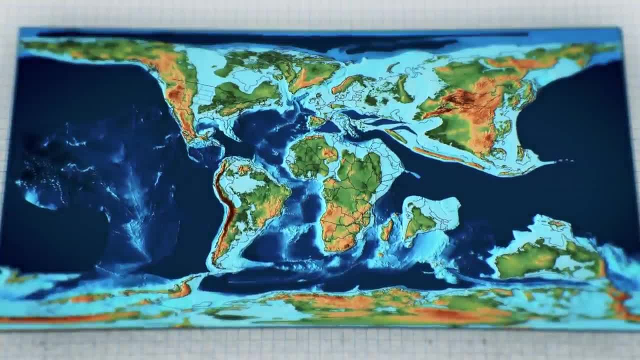 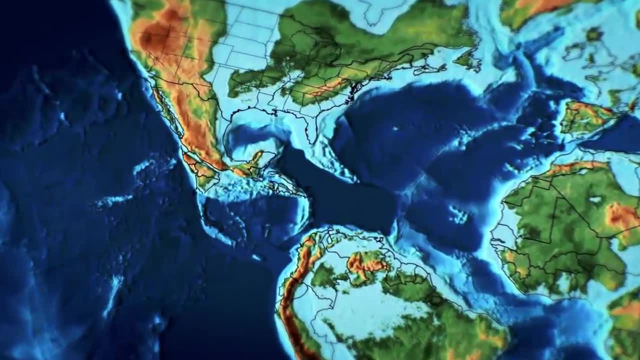 the Cretaceous period. The frame in question is this one, which represents roughly 80 million years ago. My reason for choosing this specific time is that it's the last frame in this animation before this large circular structure suddenly forms in what's now part of southern Mexico. 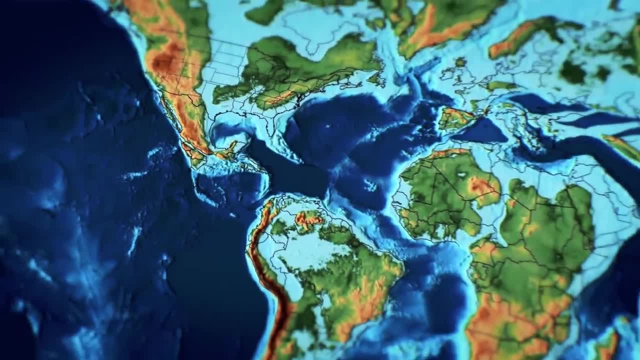 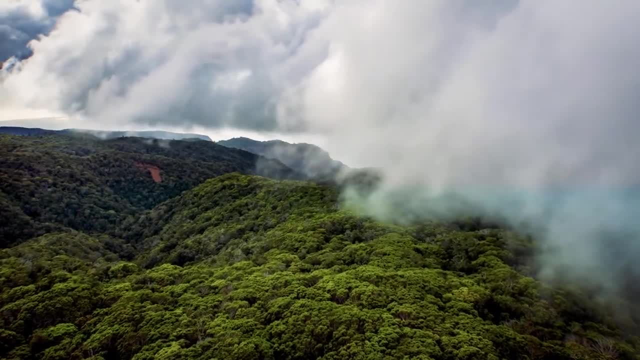 which I'll explain later why it's so important. By this point, all the continents we know today had managed to separate themselves from one another. The only thing left to do was to create a new world for the world to live in. On top of this, the exceedingly high temperatures of the late Cretaceous, combined with widespread 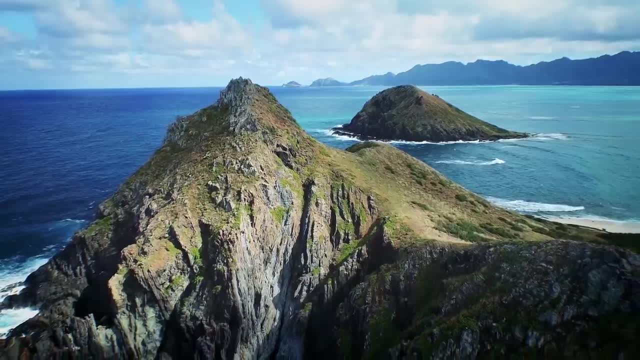 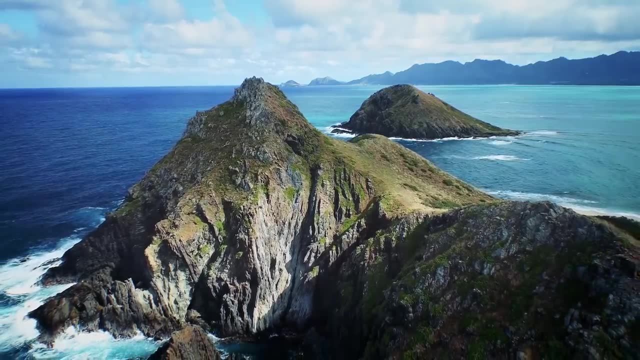 volcanism building up the ocean floor drove sea levels far above where they are now, leading to many landmasses experiencing widespread flooding across their low-lying interiors. That's how we ended up with a North America broken into three pieces, held up on the east. 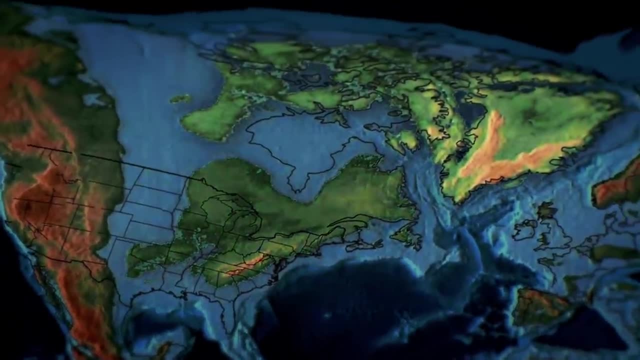 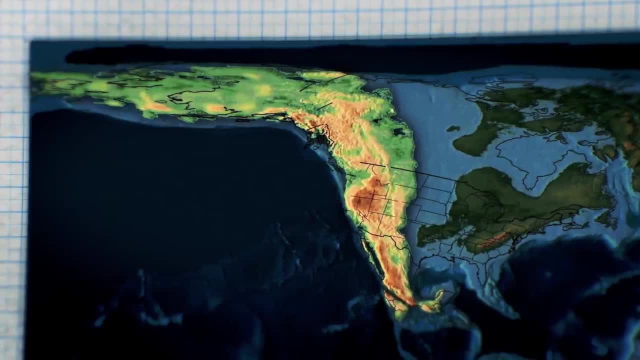 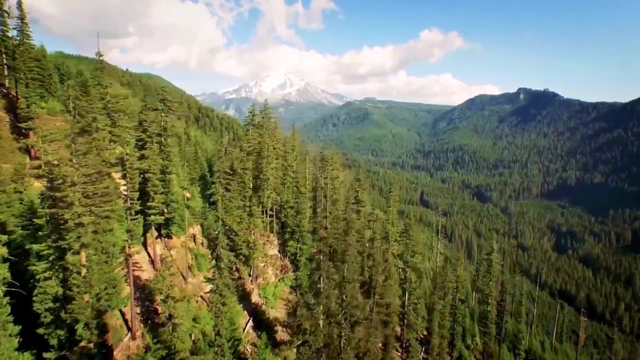 Next we have the Laramidae Mountains, which were first crossed by the Rockies, which were, at this time, entering a new phase of rapid growth, what's known as the Laramide Orogenae, or, in simple English, the Laramide Mountain Building Process, giving the landmass its 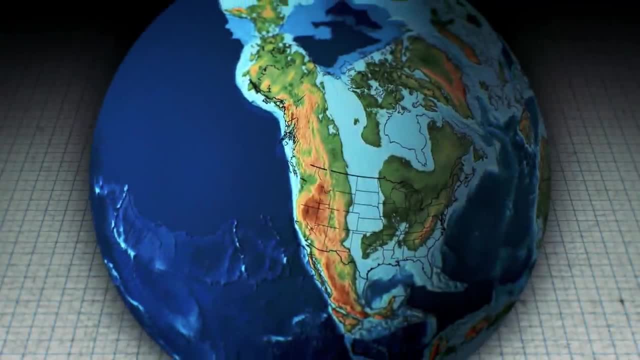 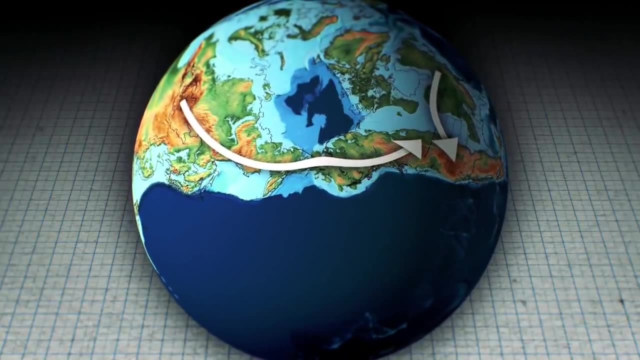 name Laramidea. Situated like this, Laramidea stood to receive genetic influx both from Appalachia as well as from Asia, positioning it to amass a huge animal community, more diverse than anywhere else in the world. Here, all of those groups of ornithischians were represented in the name Laramidia, as 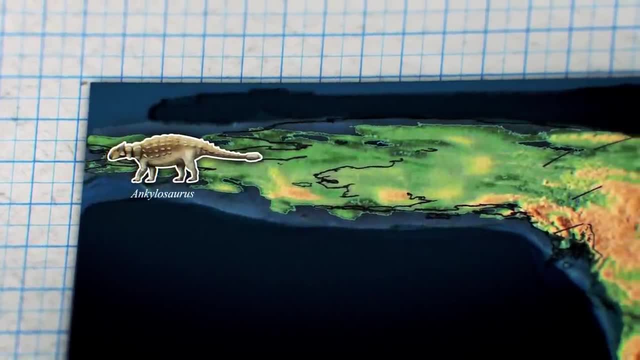 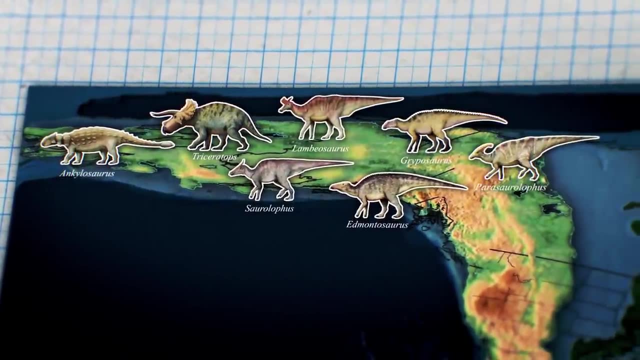 presented by ankylosaurs like well, ankylosaurus, ceratopses- like everyone's favorite- triceratops, plus many more hadrosaurs like well, take your pick. and pachycephalosaurs like well. 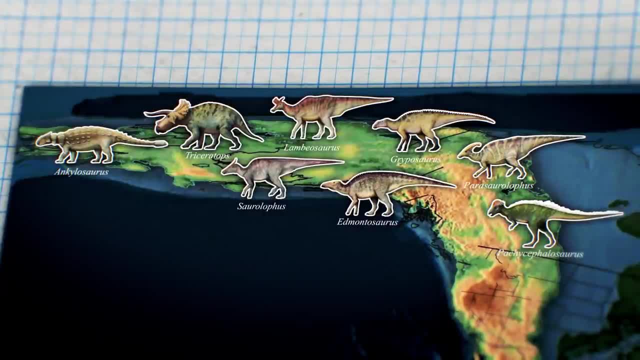 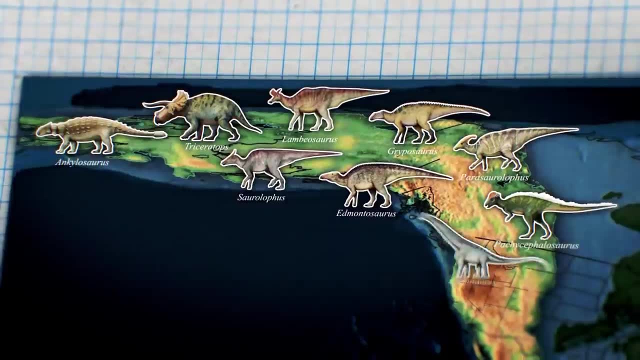 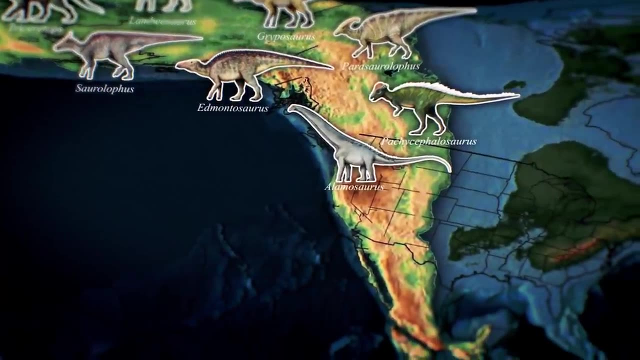 pachycephalosaurus On top of this. while the great success of the ornithischians here definitely overshadowed sauropods, this did not mean they went extinct here and were also around in forms like Alamosaurus. Between the two carnivorous theropods of Laurasia, Tyrannosaurus won out here the largest species. 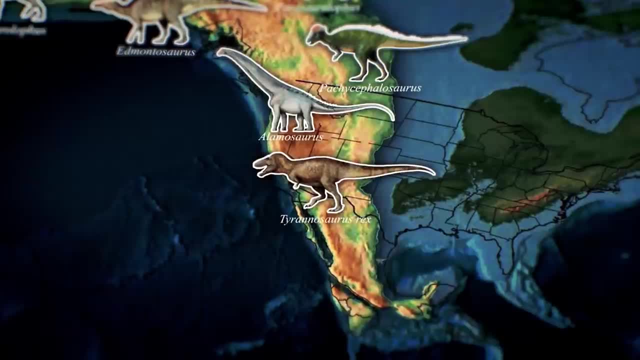 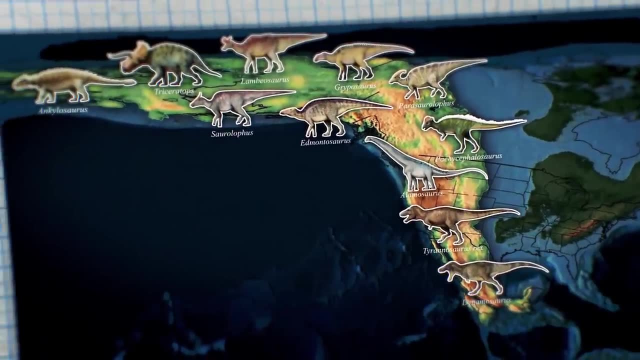 of which being, yeah, Tyrannosaurus rex, among many others, like Dynamosaurus Altogether, the fauna of Laramidia during the late Cretaceous represents the most well-known cast of dinosaurs in the world, despite, for the most part, only living here in western. 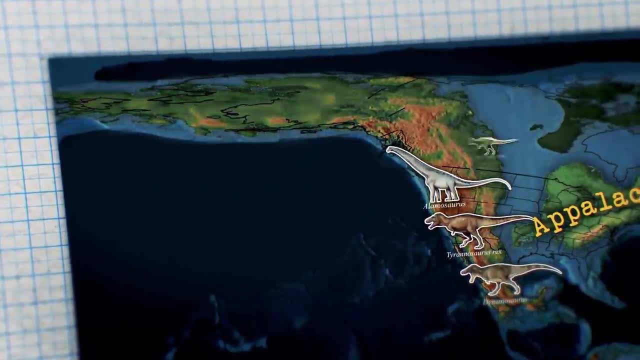 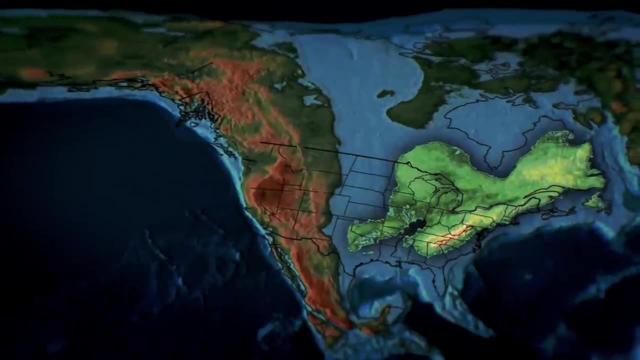 North America, Even in Appalachia, Laramidia's closest relative, both geologically and biologically. such high levels of diversity are not seen in the fossil record. While there were some Tyrannosaurids like Driftosaurus, these were all fauna. 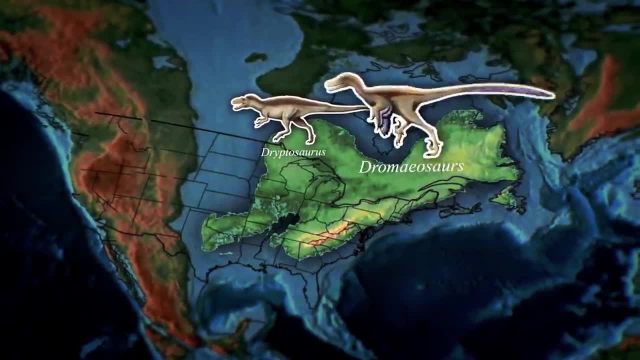 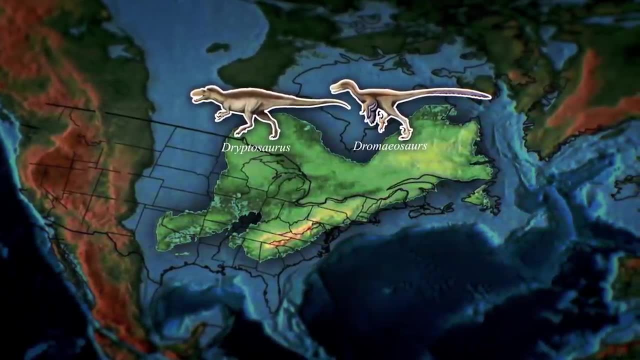 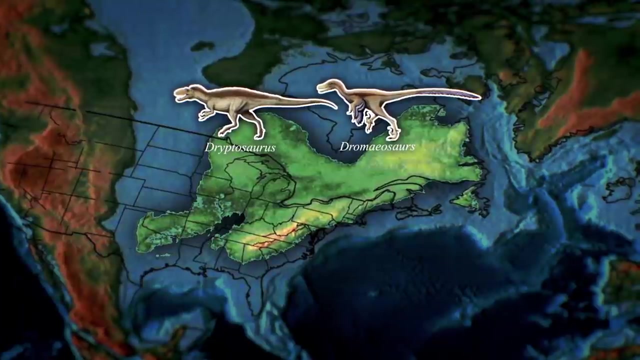 They were far smaller than their Laramidian counterparts, giving the dromaeosaurs the opportunity to share in the top carnivorous role. The hierarchy of herbivores also varied between the landmasses, with Appalachia lacking notable numbers of ankylosaurs, pachycephalosaurs and ceratopses in exchange for a more widely 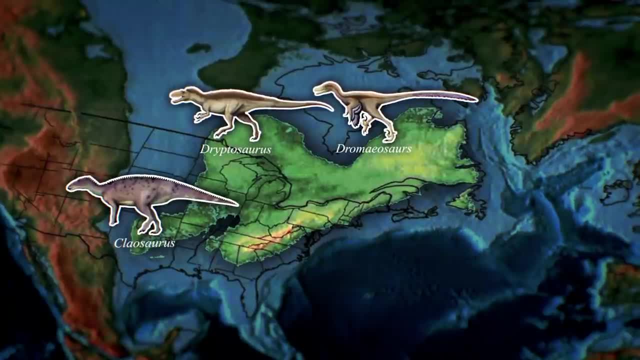 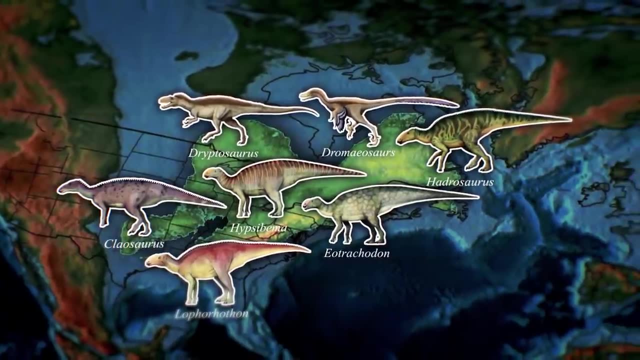 diversified group of hadrosaurs like Cleosaurus, Lopharhothon, Hypsibema Eotrachodon and, of course, Hadrosaurus. With this assortment of species, the faunal community of Appalachia more closely resembled. 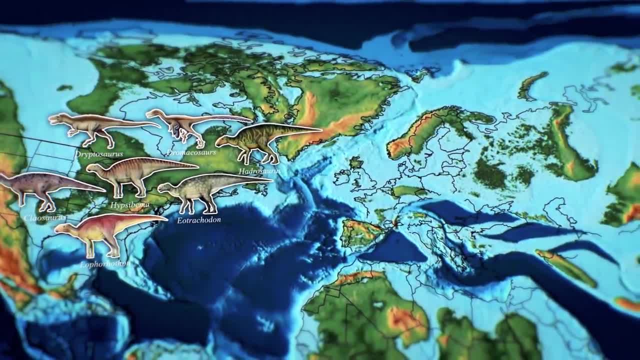 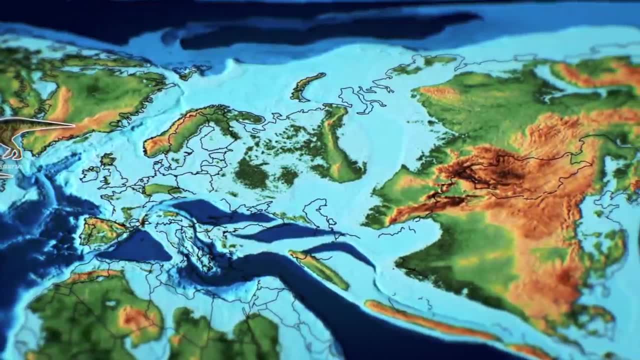 the scattered islands of what's now Europe than Laramidia, which makes sense considering their not-so-distant breakup and their isolation from Asia, due to much of what's now Russia being completely underwater at the time. And lastly, for North America, we have this northern landmass. 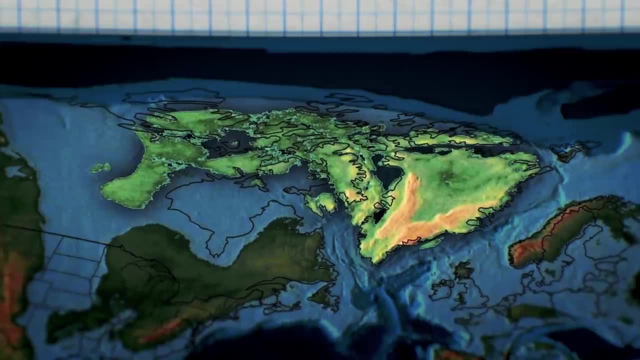 Unfortunately, we don't actually know that much about this place. Heck, I couldn't even find a name for it. I mean, going back in time, we can see that for most of its history, it was a place that was known for its natural beauty. 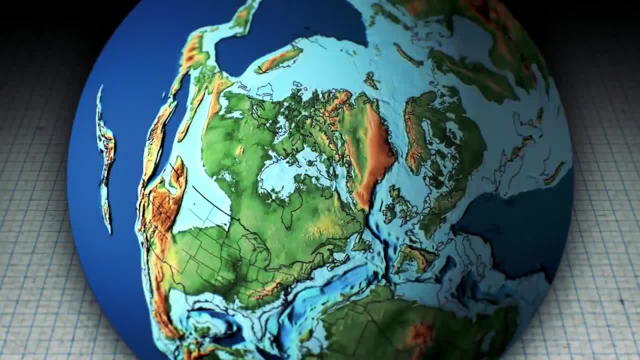 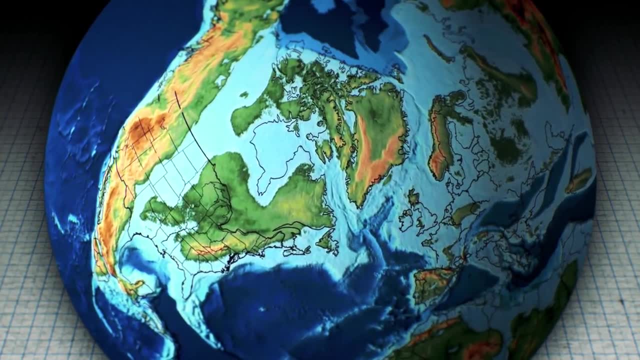 In most of its history, it was either connected to Appalachia or North America as a whole, and only appears separate in this single frame, suggesting it too would have closely resembled the animal communities of these lands, probably not even having the time to develop into its. 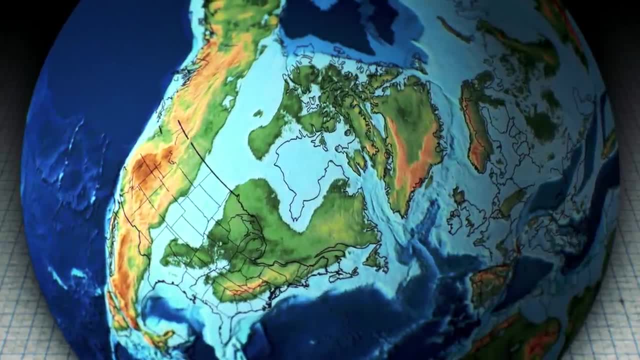 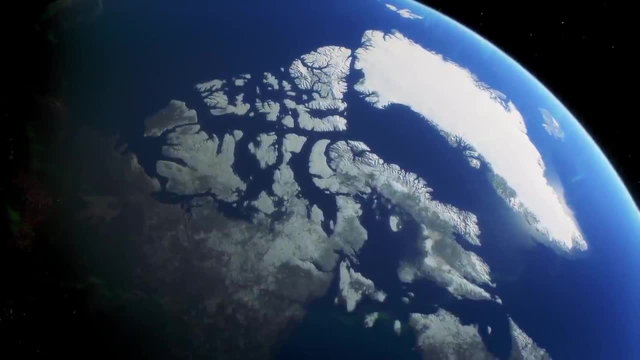 own distinct biota, but rather belonging to the greater Appalachian realm. But here's the thing: we really just don't know. Fossil discoveries from this part of the world are scarce, partially due to the fact that barely anyone lives here now. 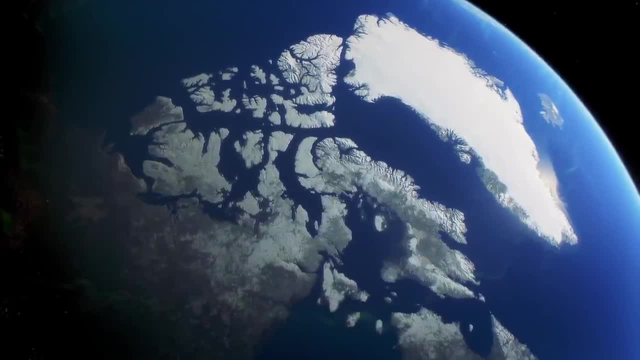 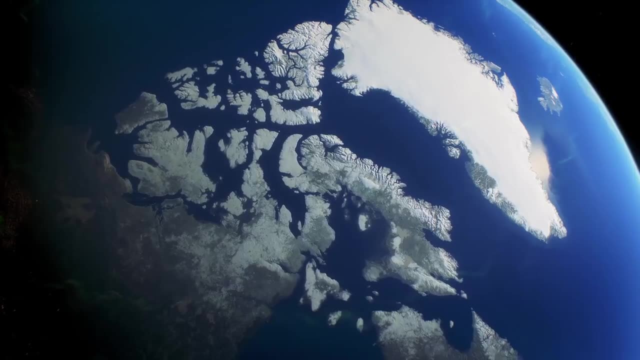 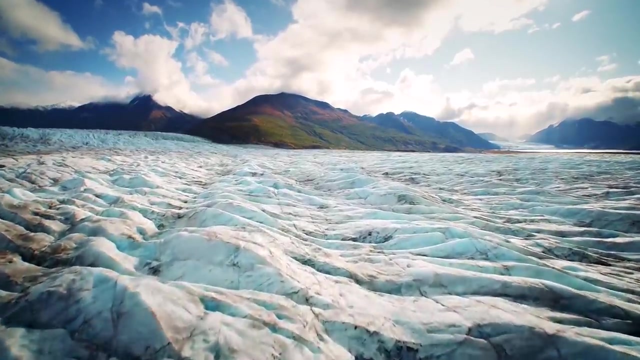 But even more so because of what these lands experienced only a few thousand years ago, having been covered in massive ice sheets several times over, with Greenland even remaining covered to this day. The destructive nature of these glaciations have, in effect, erased much of the fossil record. 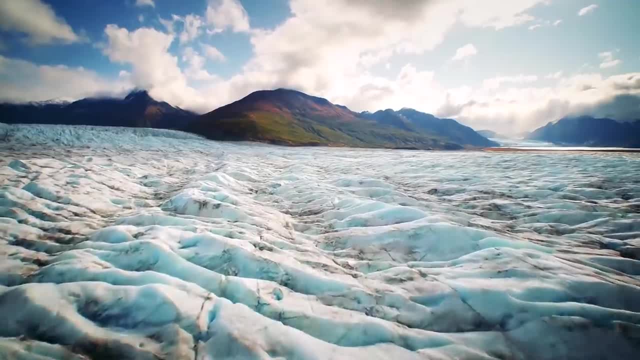 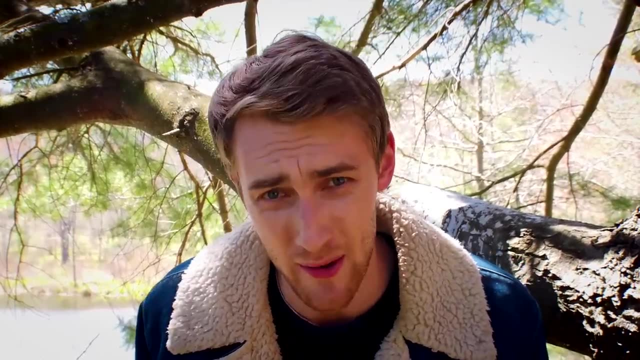 here, meaning we can only guess as to what the species makeup of this land was. Given the brief history of this landmass and the lack of fossil specimens, not much more can really be said about it. But don't worry. In a world like paleontology, knowing what you don't know is equally important, if not. 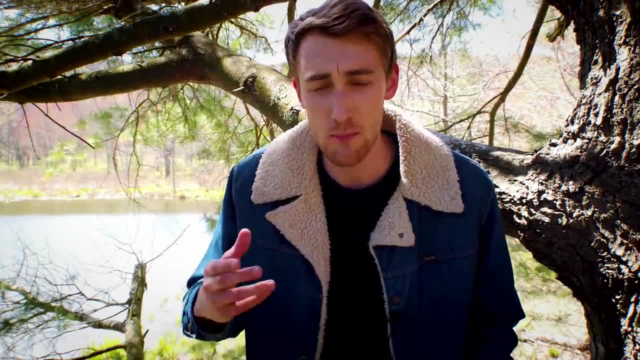 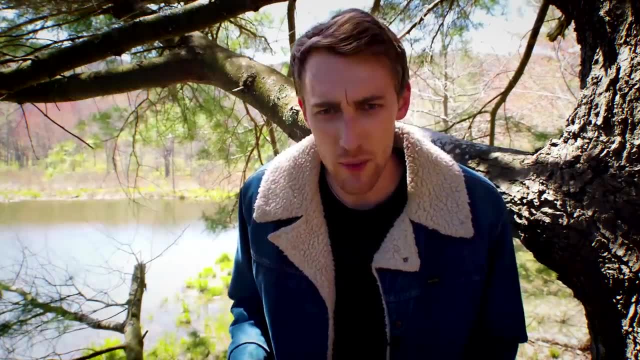 more important than knowing what you do know, As the only way to make a discovery is by taking something from the unknown into the known, and to do this you need to know where to look. But even without knowing much about this one landmass, the picture that's emerging is: 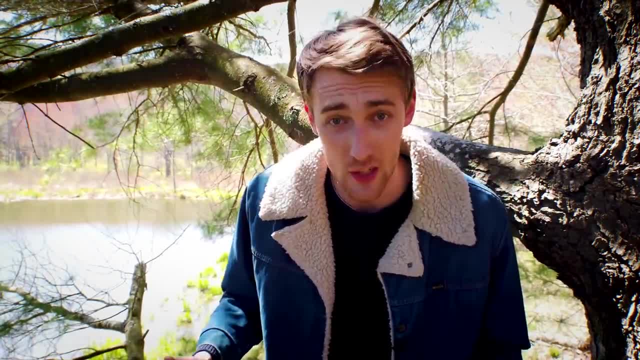 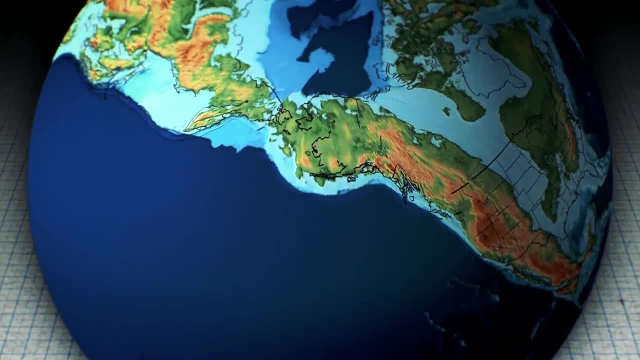 one of a North America that hosted a highly diverse ecosystem. Okay, where were we? Oh, that's right. looking back to Laramidia, we can see that it was actually in closer contact with the Northeast- It was east of Asia at the time, with the two continents even periodically reconnecting. 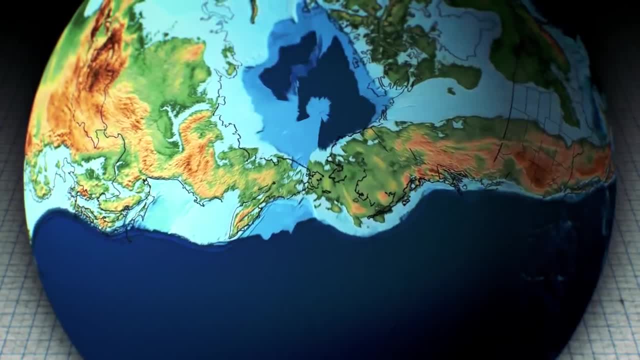 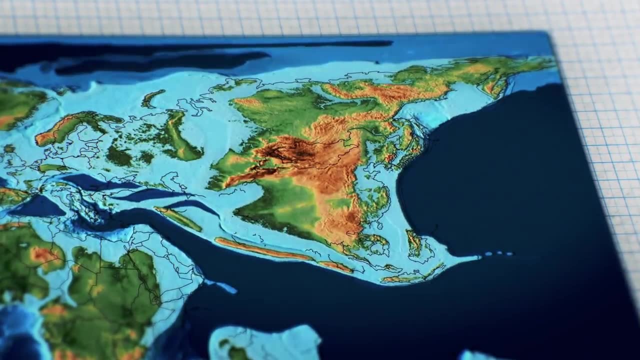 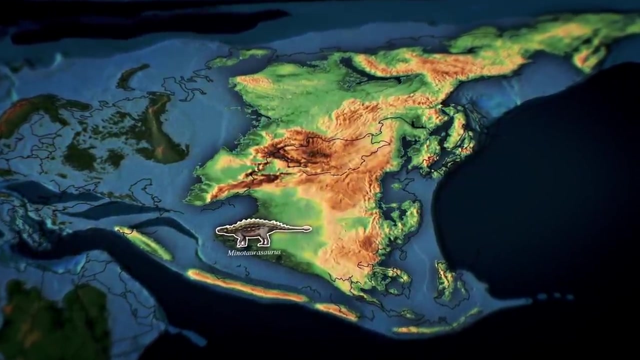 to each other, sometimes for tens of millions of years, leading these two lands to share in an apparently closer relationship than with Appalachia. This explains why it was here that we'll find a similarly diverse ornithischian fauna, consisting of ankylosaurs like Minotaurosaurus, ceratopses like little protoceratops and more. 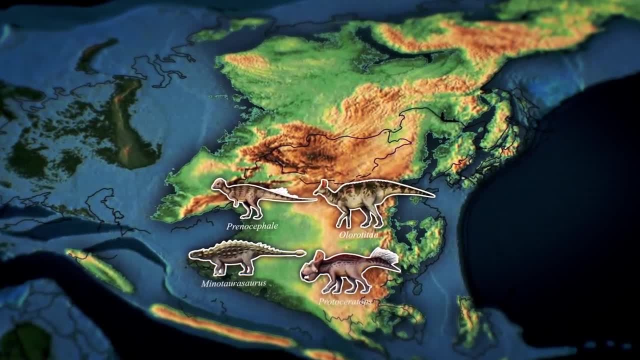 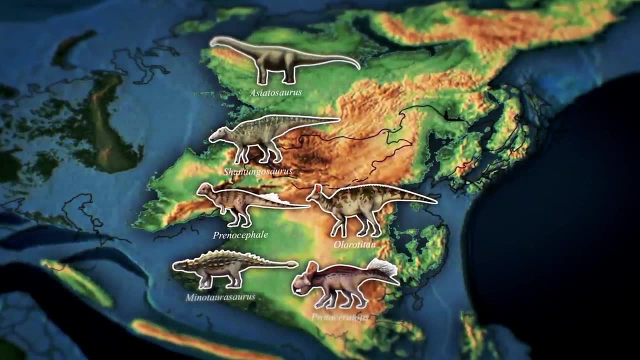 pachycephalosaurs like Prinocephaly, hadrosaurs like Olorotitan and Shangtungasaurus, along with, sure, even some sauropods like Asiatosaurus, All of which were, yes, being hunted primarily by Tyrannosaurs, though these two were smaller. 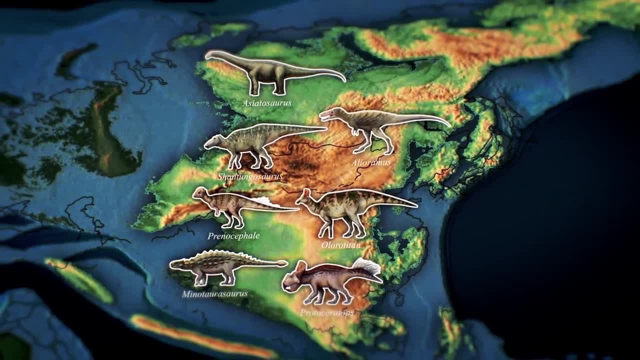 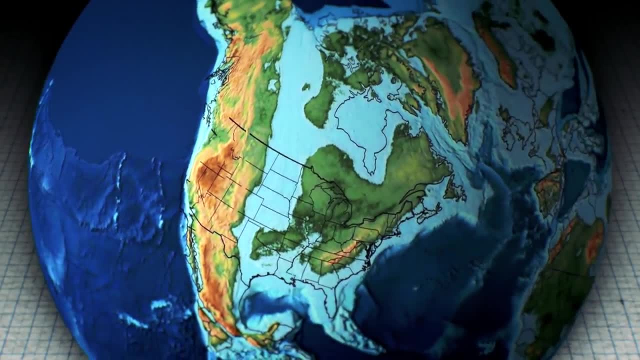 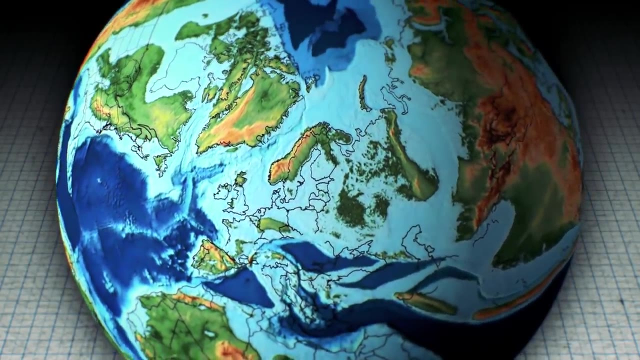 than their Laramidian counterparts, coming in the form of Allioramus, Jucheng, Tyrannus and Tarbosaurus. Looking at these three or four continents, we can already see the biogeographic realms of today taking shape, evolving apart from one another, while simultaneously remaining 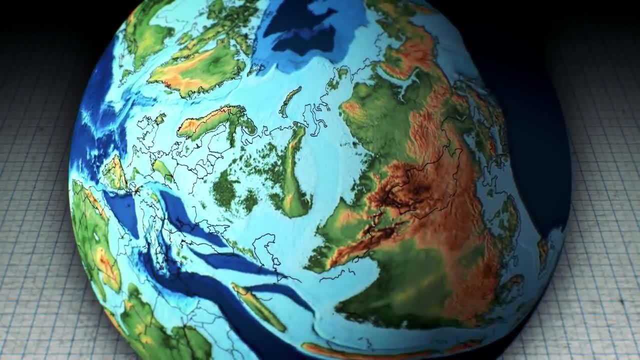 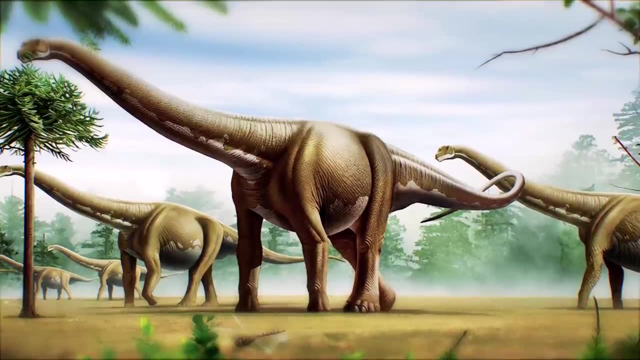 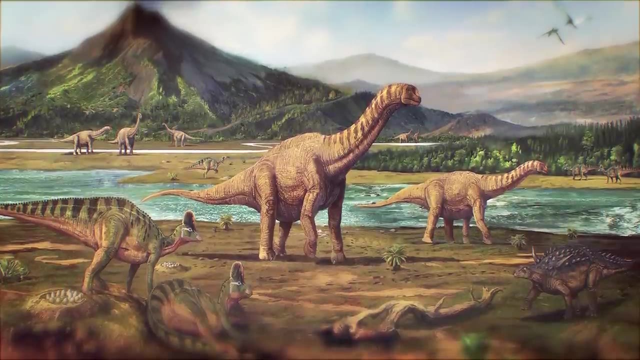 more related to each other than the rest of the continents. further south, If you'll remember, across the Gondwanan lands it was the sauropods that managed to outcompete most ornithischians for herbivorous dominance. As a result, the incredible diversity of ornithischians in the north was not present here in the south. 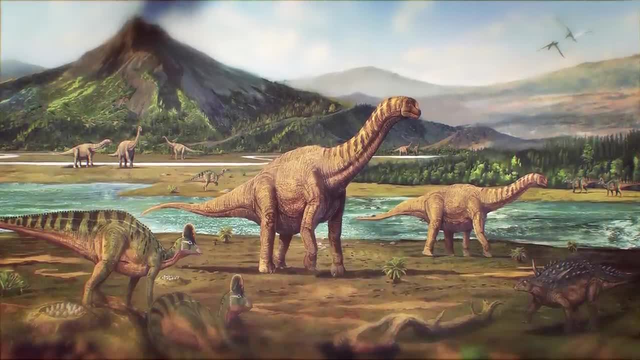 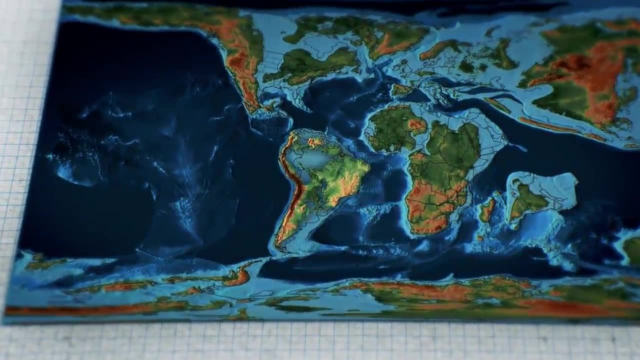 but rather we'll find many different, though let's be honest to the untrained eye: identical sauropod species Across South America, for example, which had just barely managed to stay in one piece and played host to a tremendous inland sea. 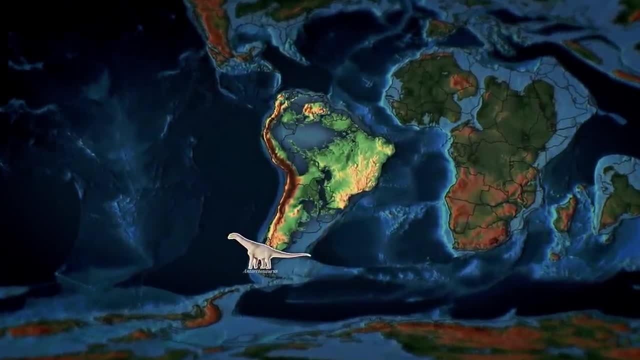 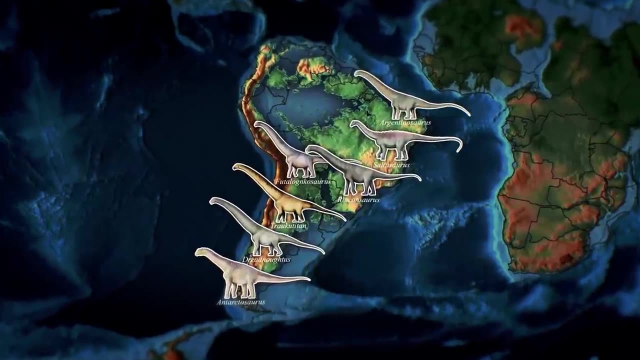 A large number of sauropods like Antarctosaurus, Dreadnoughtus, Tralcutitan, Feudalancosaurus, Ranconosaurus, Saltosaurus and, the biggest of all, Argentinosaurus, roamed, while the ornithischians 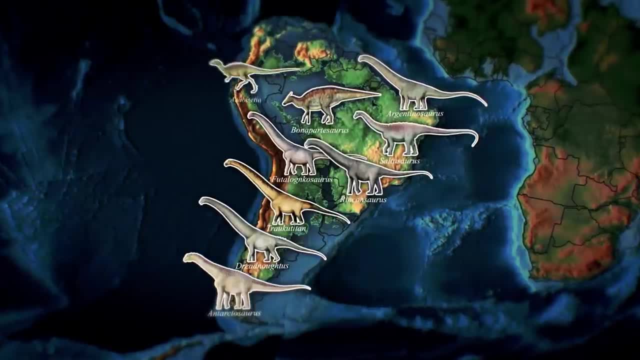 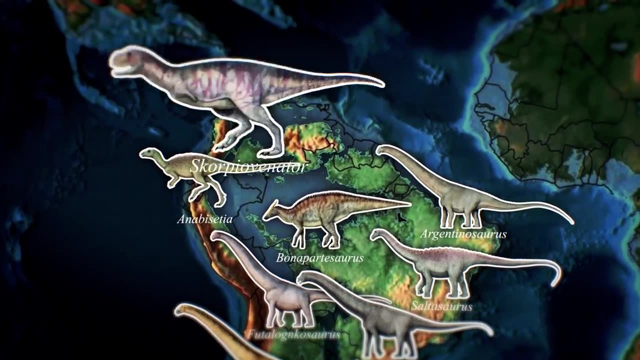 were only represented by a handful of Hadrosaurs and Iguanodons Hunting. these were not Tyrannosaurs or even Dromaeosaurs, but their theropod cousins, the Abellosaurs, like Scorpiovinotaur and Carnotaurus. 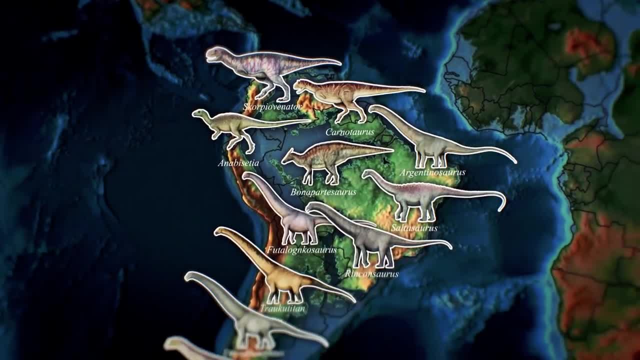 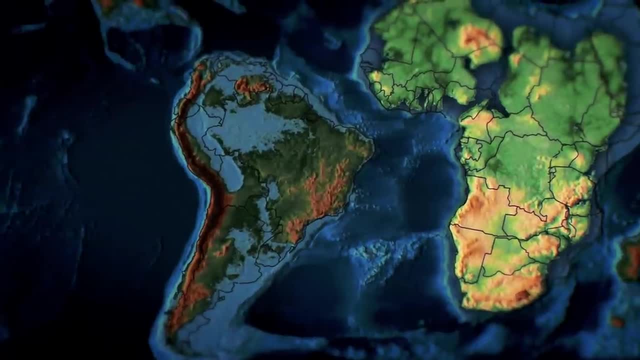 We can think of this as the blueprint for all of the animal communities across the Gondwanan. The continent was divided into two main continents: the Anduanan Continent, like Africa, which had only been separated from South America for 20 million years at this point, leaving the 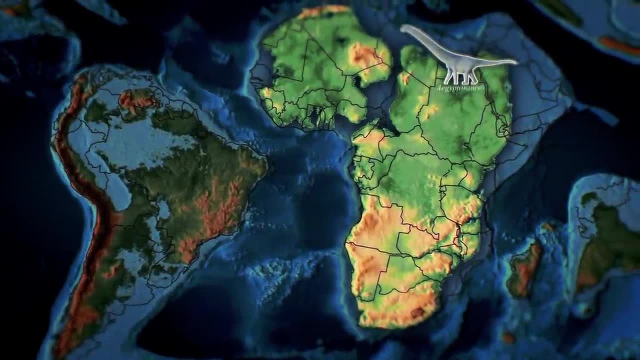 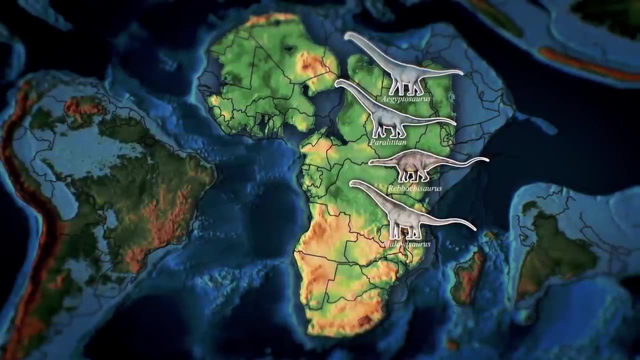 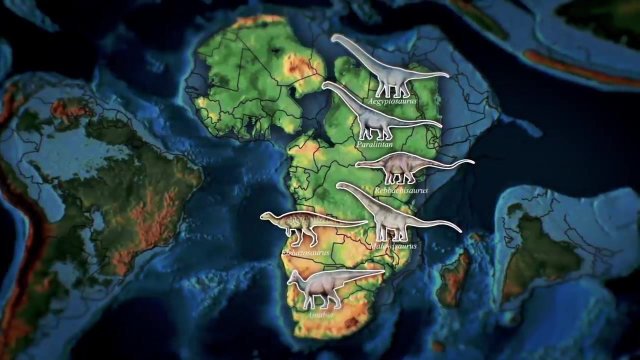 continent, with a familiar diet of sauropods like Egyptosaurus, Paralytitan, Ribocosaurus and Mollewosaurus, along with a reduced selection of ornithischians, again limited to Hadrosaurs like Ajnabia and Iguanodons like Elrasosaurus, all being preyed upon by Abellosaurs like 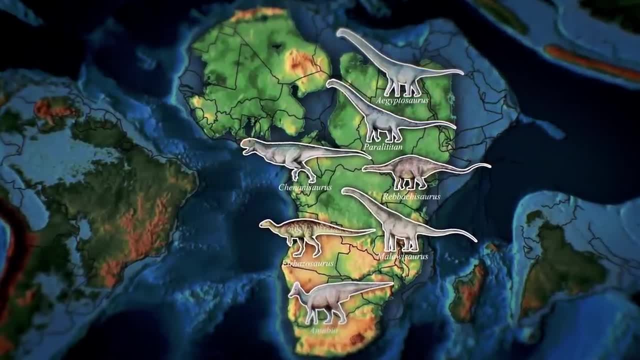 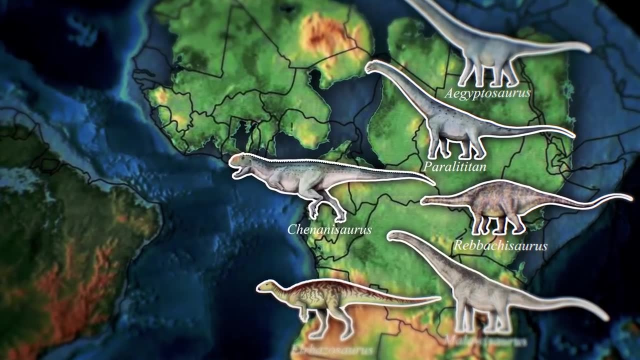 Chinannosaurus. But here's where things get interesting, The Theropods of the African realm having been locally usurped by even larger theropods known as Spinosaurus, with members like Sigilmasasaurus and, yes, Spinosaurus. 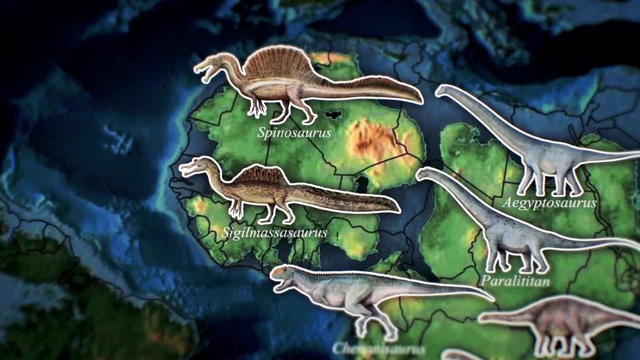 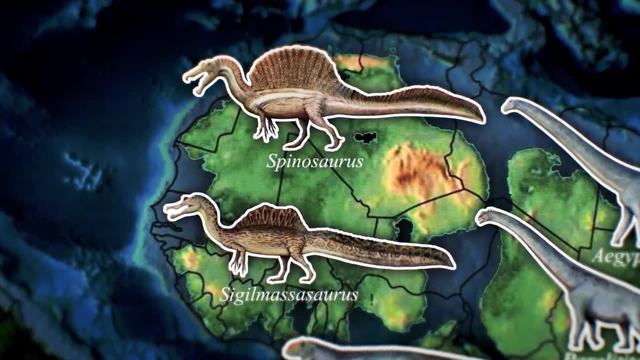 Estimated to have been potentially bigger than even a T-Rex. answers as to how Spinosaurus got so big can also help explain why they look so different from the other theropods we've seen so far. You see, Spinosaurus were believed to have been partially aquatic creatures, with their 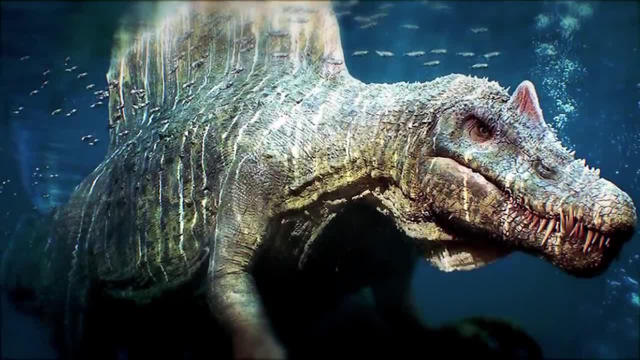 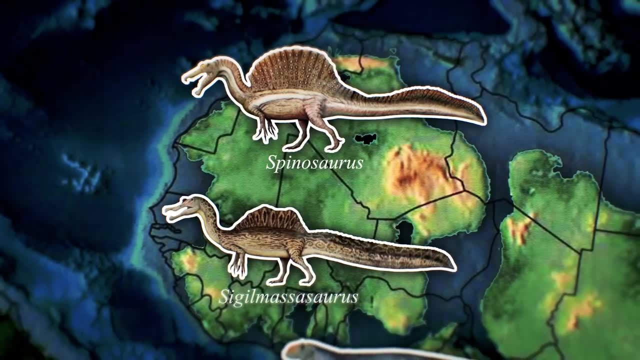 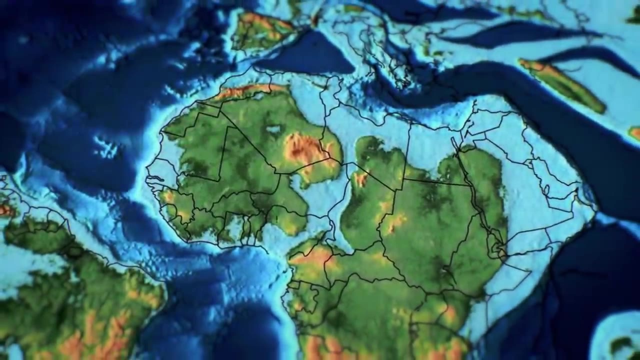 buoyancy in water, helping to take some of the weight off, allowing them to grow bigger and selecting for more muscular tails to help them paddle through water. A potential reason these theropods evolved into the water could be that, similar to North America, Africa was also fractured as a result of the particularly high sea levels of the. 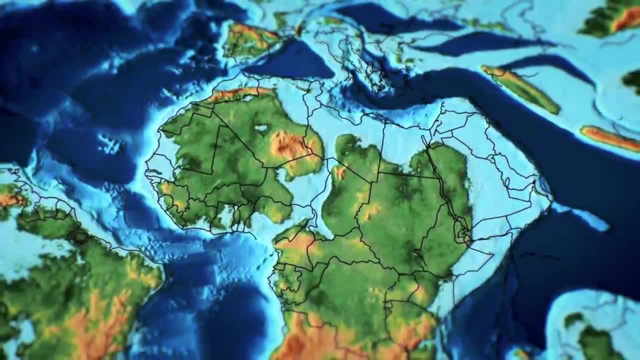 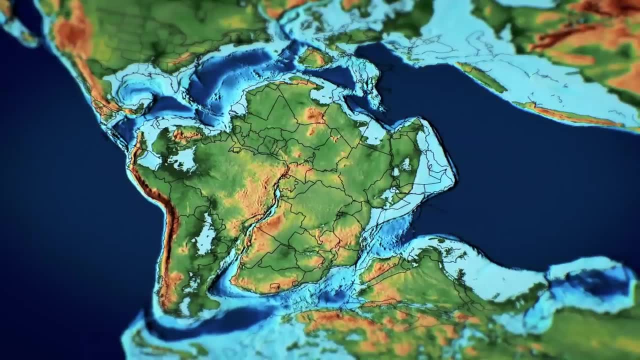 time, with a narrow and shallow inland sea crossing between east and west. Having formed nearly thirty million years prior, this divide between the Theropods of the African realm and the Spinosaurus was a major factor in the development of the continent. This divide between the two halves of the continent was present for nearly the same. 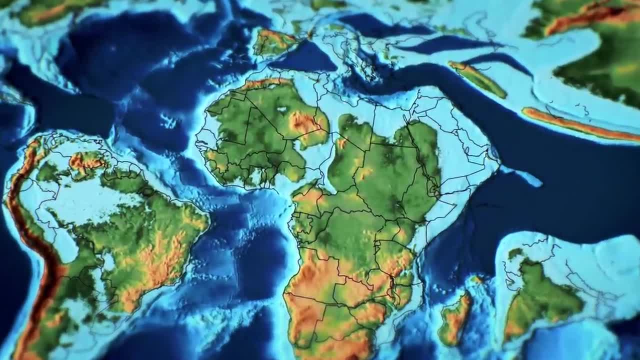 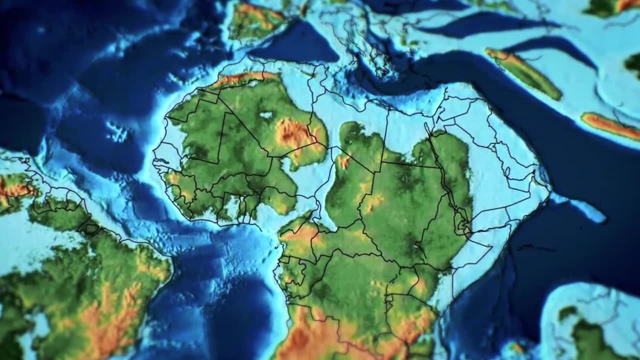 amount of time as the western interior seaway that split Laramidia from Appalachia, suggesting the possibility that these two landmasses could have formed their own distinct realms for a time. But to be honest, I just couldn't find enough evidence to support this. 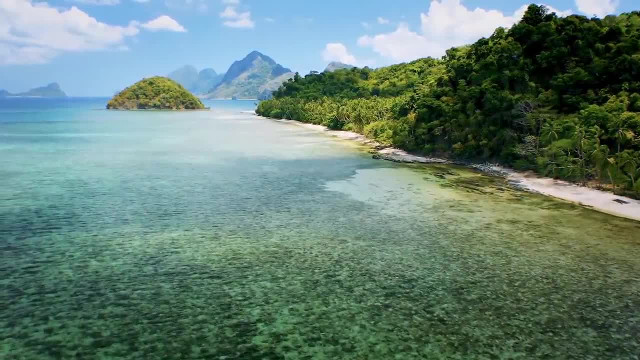 Perhaps the narrower inland sea allowed for easier crossing between the two African fragments, or perhaps the sea was shallow enough to form temporary islands. Or perhaps the sea was shallow enough to form temporary islands. Or perhaps the sea was shallow enough to form temporary islands. 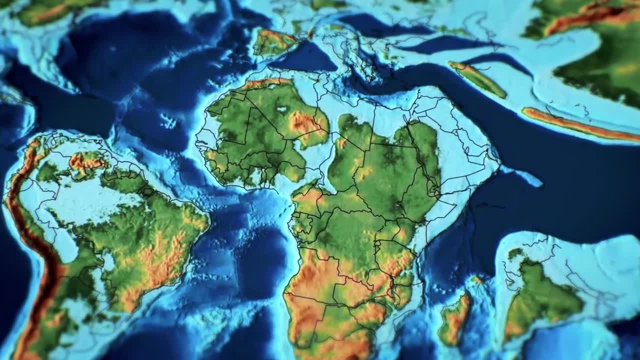 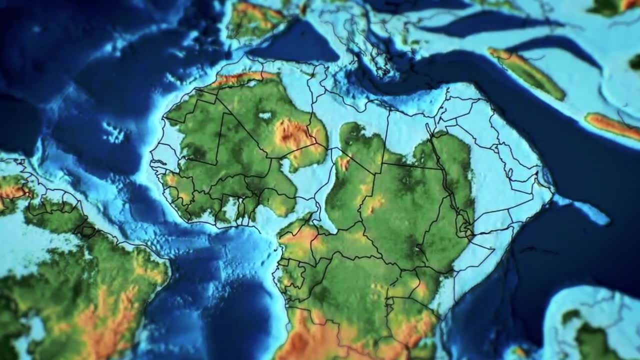 Or perhaps the sea was shallow enough to form temporary land bridges, Or, and in my opinion most likely, perhaps just not enough fossils have been found in Africa to actually help us differentiate the two lands. yet The fact of the matter is is that while dinosaur mania swept through North America, fueling a huge number of discoveries, even something called the Bone Wars. Africa, at the very same time, was being colonized, and well, it wasn't fossils that the colonizers were after, Leaving many places like Africa and elsewhere around the world drastically isolated from. Africa drastically understudied. I mean, just look at how short the list of known African dinosaurs is compared to the list of known North American dinosaurs. It could very well be that we just have more data on places like North America and Asia and with time, as more details are uncovered and discoveries made in places like Africa, the big picture could change Or not. I don't really know, but that's part of the beauty of paleontology: We're not even close to knowing all the different genuses of dinosaurs, let alone species and all it. 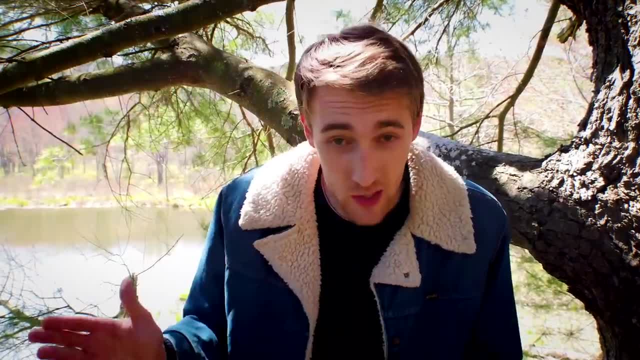 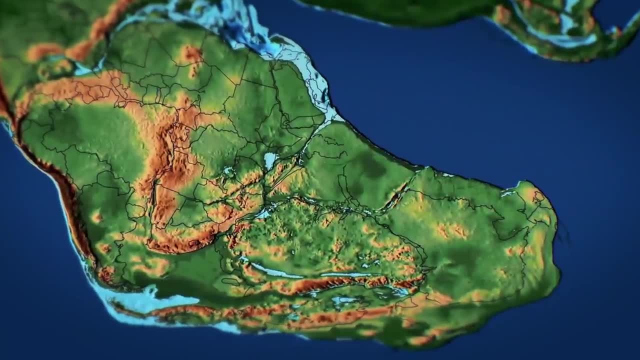 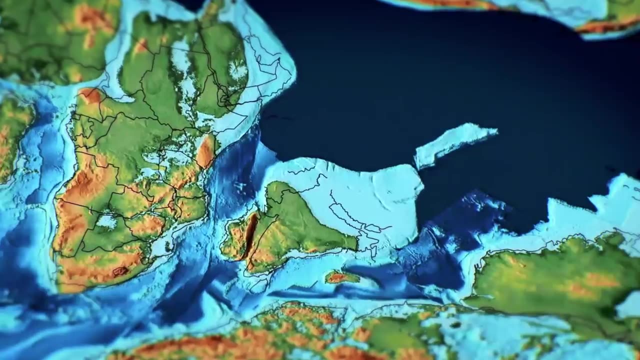 would take is a handful of dedicated scientists to completely alter our understanding of them here. The story is again the same for India and Madagascar. It was together that these lands broke from the rest of Gondwana forty million years before our final map, and only separated from each other 20 million years later. 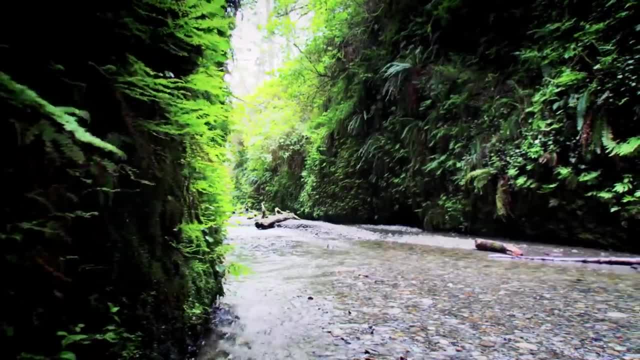 This means that, while potentially enough time had passed for the fauna of the two landmasses to have diverged slightly from other gondwanan animals, not enough times for the species to have赴a的時候 sushi species to be built up. 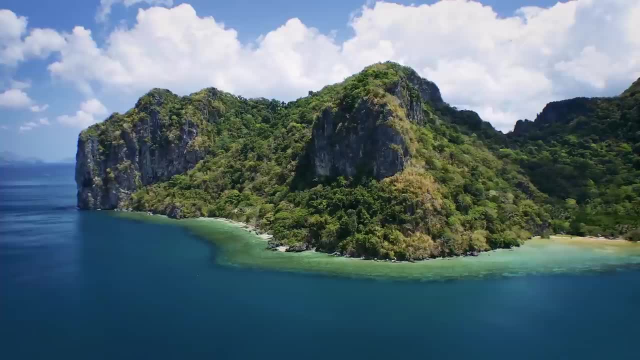 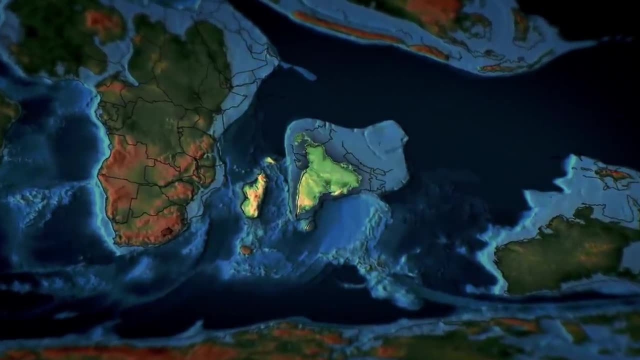 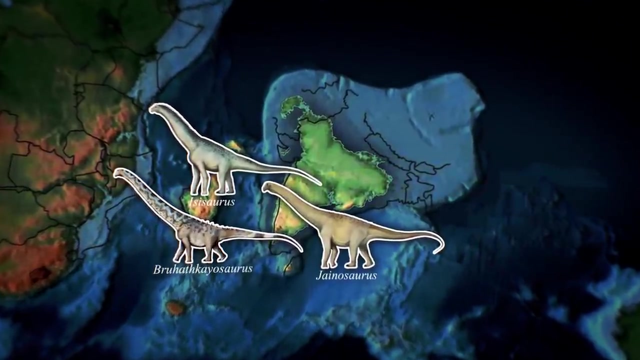 time had passed for any significant difference between them to be found in the fossil record, and so they could still be considered a single combined realm. Unsurprisingly, here we'll find a classic Gondwanan animal community, where sauropods like Brahatkaosaurus, Isosaurus and Janosaurus served as the only known herbivores during. 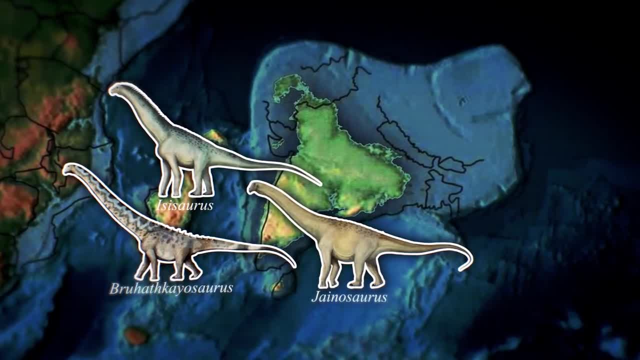 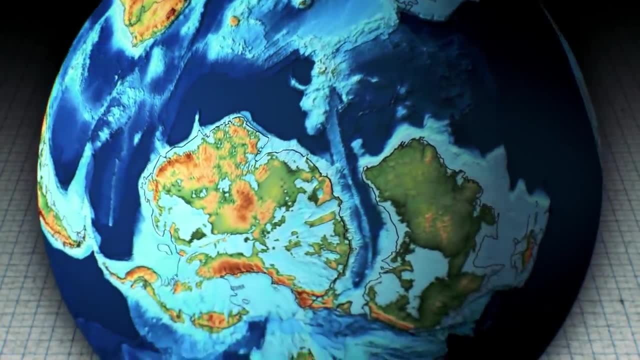 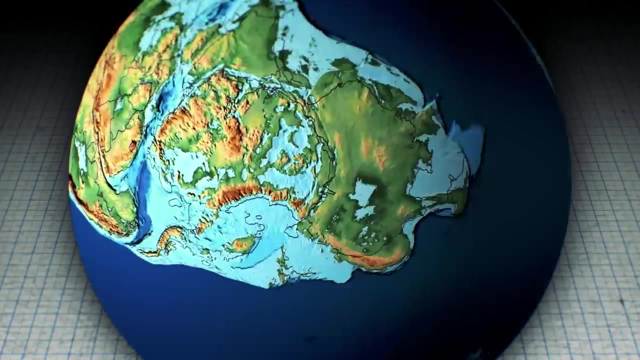 the late Cretaceous, all being preyed upon by abelosaurus like Rajasaurus and Majungasaurus. Finally, this brings us to the southern continents of Antarctica and Australia, which had also been combined, for most of the dinosaurs reign on Earth and were only in the early stages. 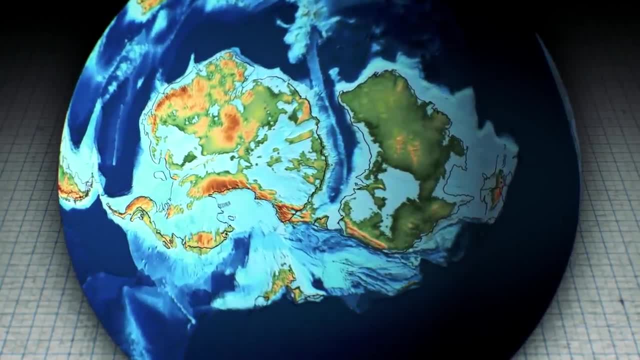 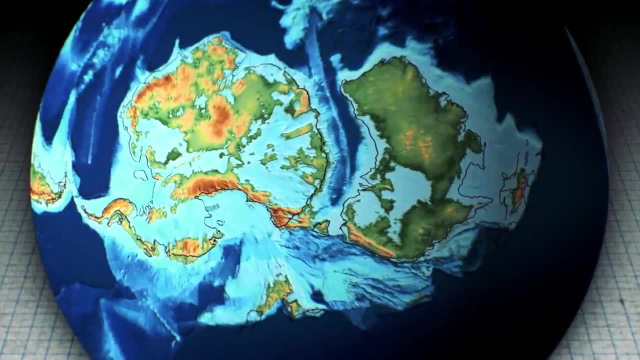 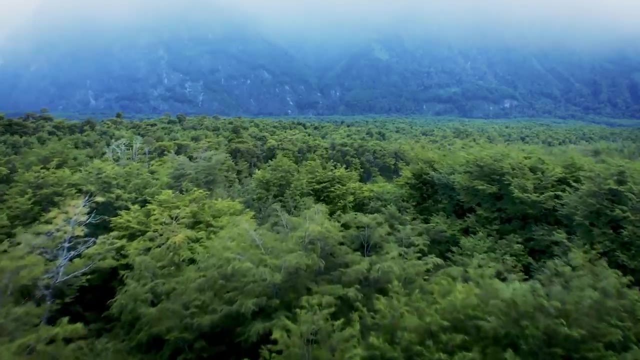 of breaking apart by this time, Like India and Madagascar. the recent attachment of these two continents means their related animal communities could not have substantially diverged from one another yet, and the lands could have been considered under a single australic realm, Unlike today the south pole of the Cretaceous. 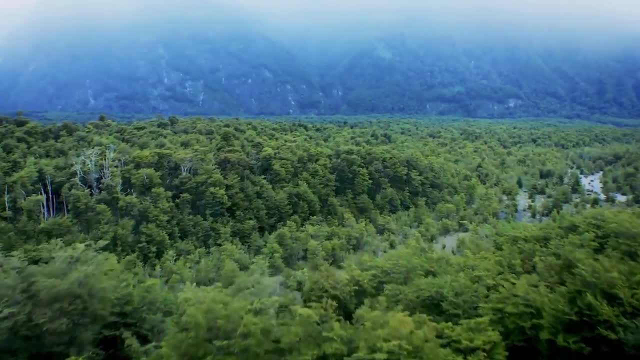 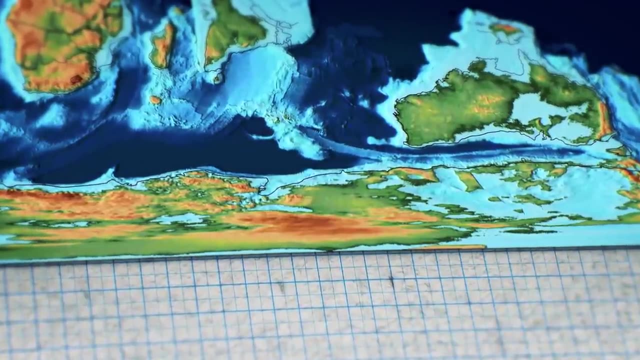 was bathed in the excess heat of a greenhouse earth, allowing forests to cover the two continents wherever there was enough water to do so, in turn sustaining communities of sauropods like Diamantinosaurus and Savannasaurus, alongside a small selection of Ornithischians with 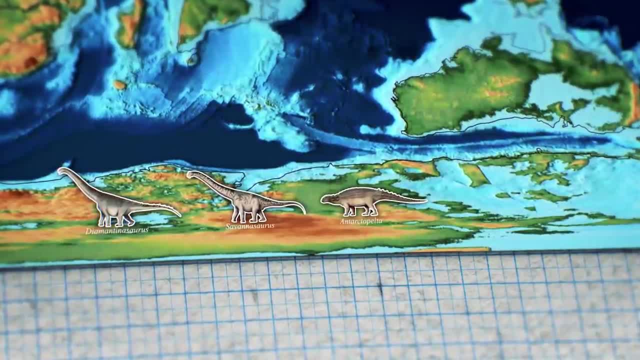 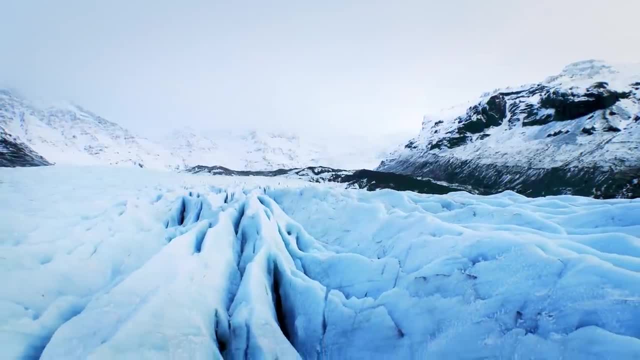 Ankylosaurs like Antarctopelta, and Iguanodons like Trinosaurus and Morosaurus. However, since then, huge ice sheets have piled on top of the land, making recovering most Antarctic fossils impossible, leaving the fossil record for this southern realm. 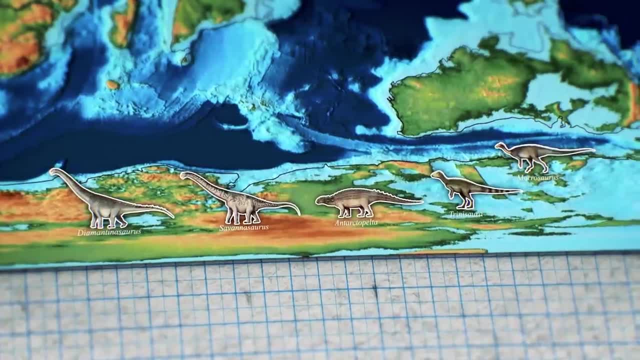 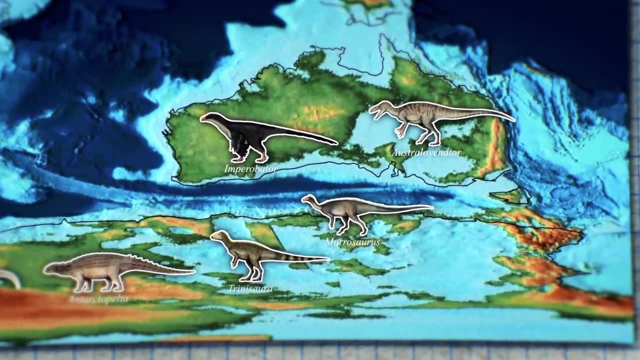 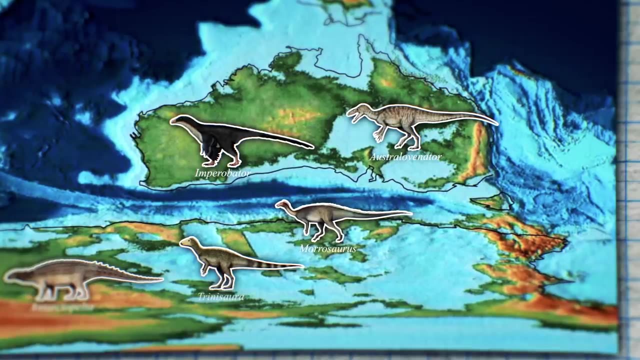 far more incomplete than any other. As such, the only carnivorous dinosaurs known to have lived here during the late Cretaceous were Imperobiter and Australovenator, both only small to mid-sized theropods that were likely not the true apex predators of the southern lands. 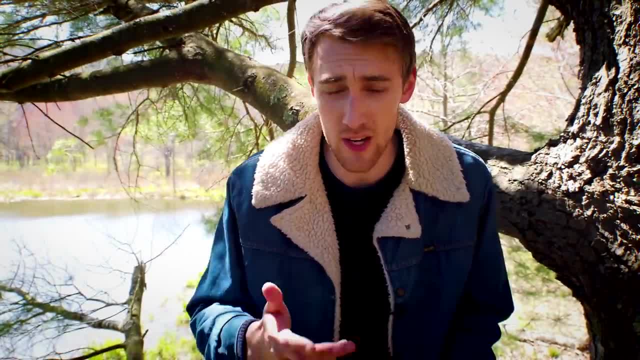 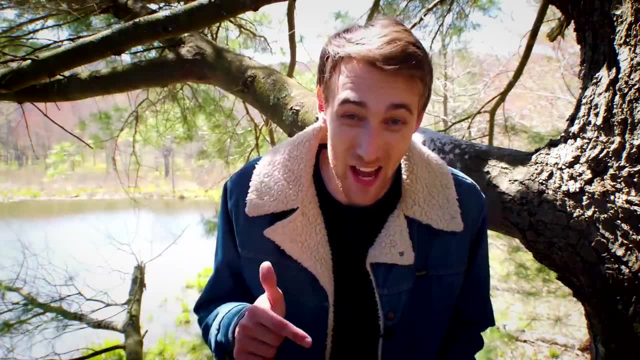 Altogether. what we can see from this is that, while the specific species of a continent varied, they all followed the same structure, The structure that was established all the way back in Pangea. As it stands now, it appears that dinosaur diversity peaked in the western half of North. 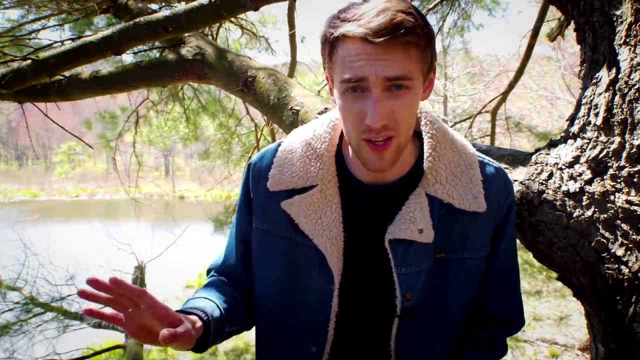 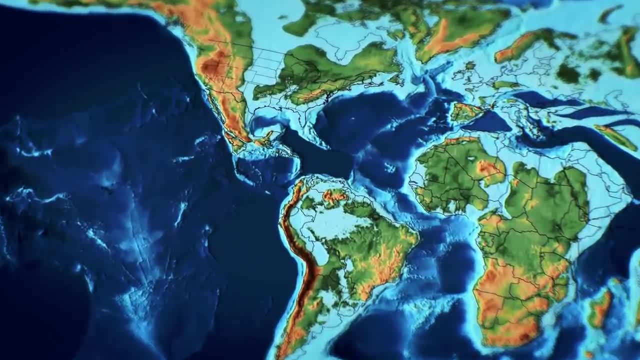 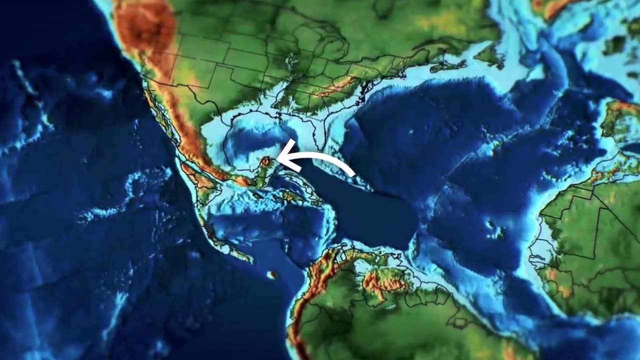 America, though in time, the dinosaur communities of all the continents could have diversified to a similar degree. Except, as we all know, the time of the dinosaurs was cut short as just a single frame forward. and again this small circular feature appears towards the south end of Laramidia. 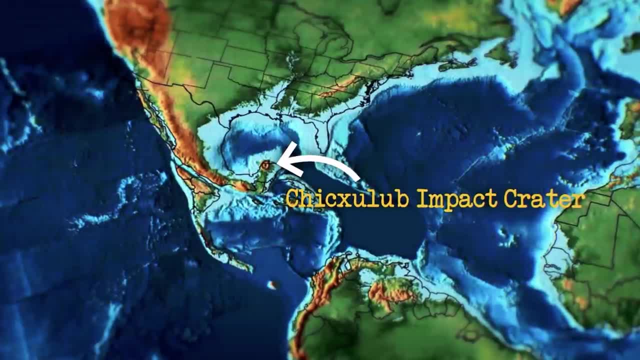 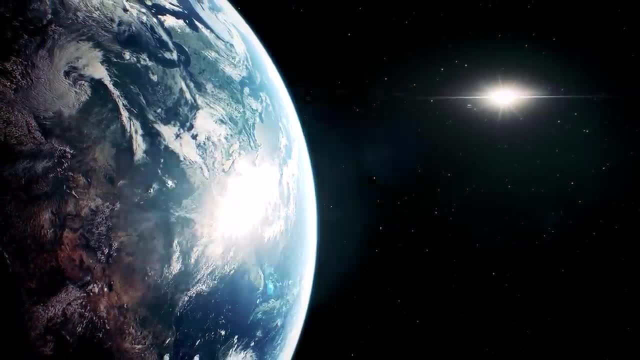 This is the Chicxulub impact crater. This crater was created 66 million years ago, when an asteroid 6 miles in diameter came crashing into the earth, putting an abrupt end not only to all of the dinosaurs mentioned in this video, but also to the Cretaceous period as a whole. 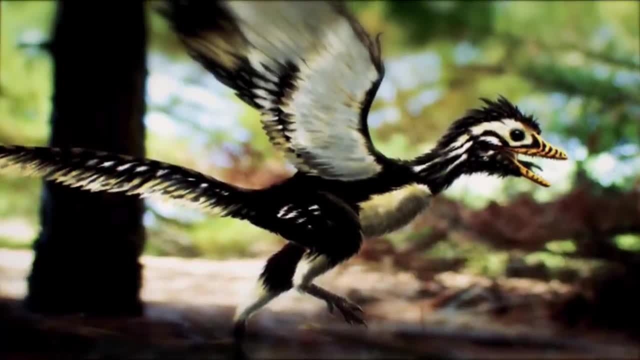 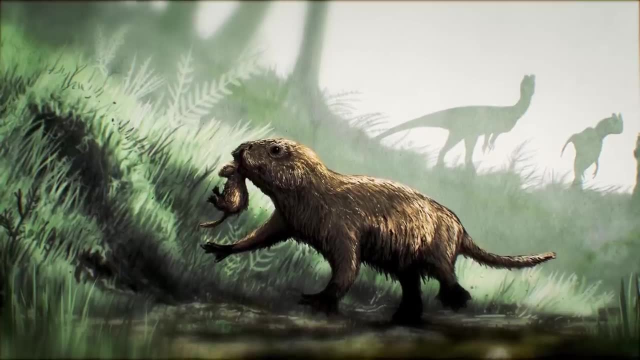 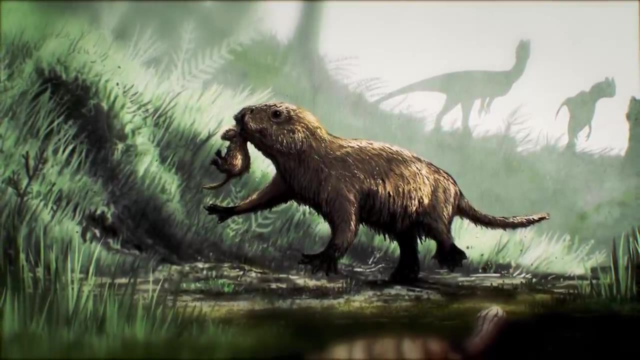 The only dinosaurs to survive this event were a small group of theropods known as the avians, the ancestors to all modern birds. But, lucky for us, life is never done evolving, and the extinction of the dinosaurs left a hole in the earth's ecology that would eventually come to be filled by mammals.